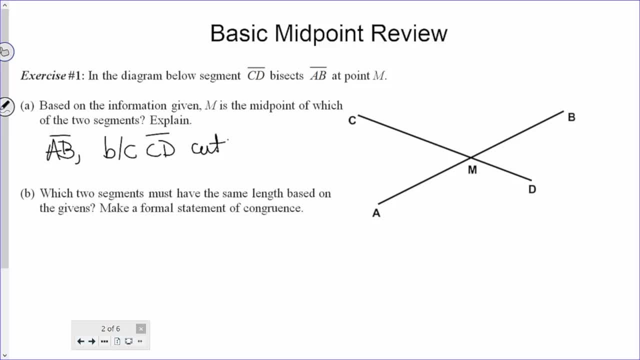 see M cuts AB in half right. CD is the bisector of AB, right, Great Easy enough. Letter B, Which two segments must have the same length based on the givens, Make a formal statement of congruence. So do that. Which two segments in this diagram, based on the fact that N is: 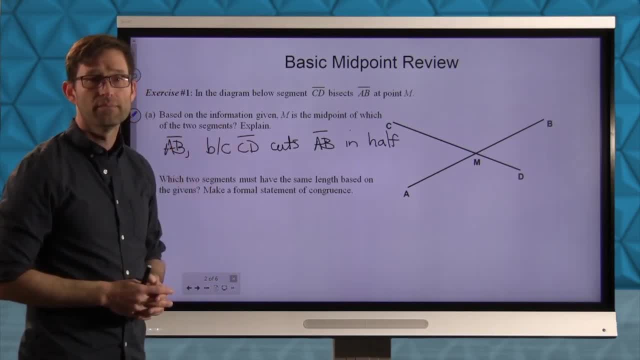 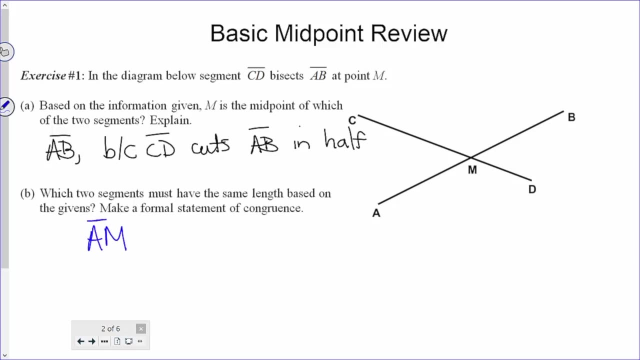 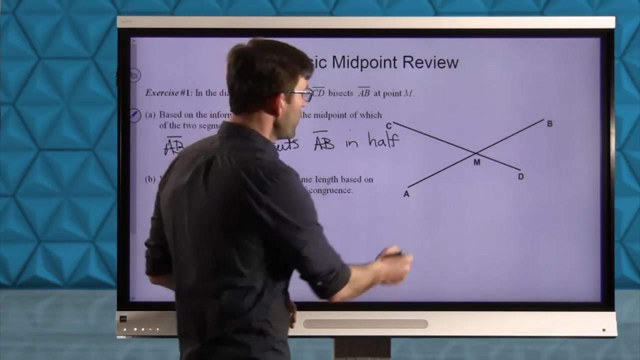 the midpoint of AB have to have the same length, Alright. Well, that would be: a? n right must be congruent to b? n. Alright, These two have to have the same length because that is the definition of a midpoint. 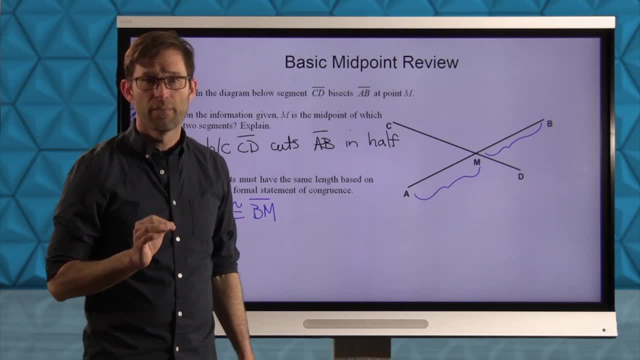 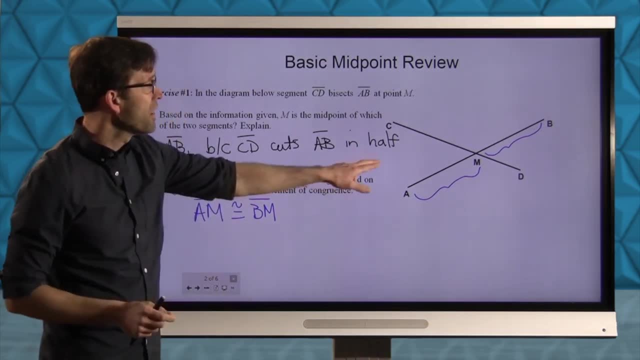 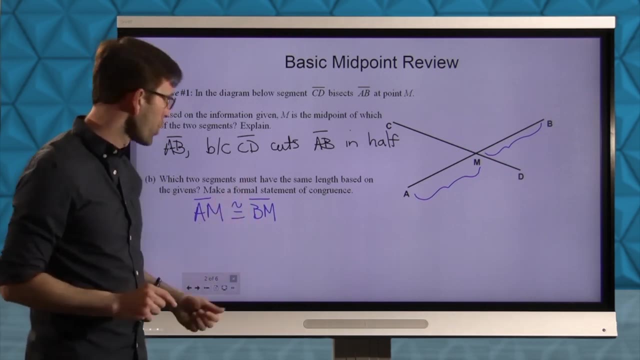 A midpoint is that one unique point on a line segment that divides it exactly into two congruent segments, two segments of equal length. Those two happen to be a, n and b? n. Alright, So simple enough. Let's now look and move to the coordinate plane. 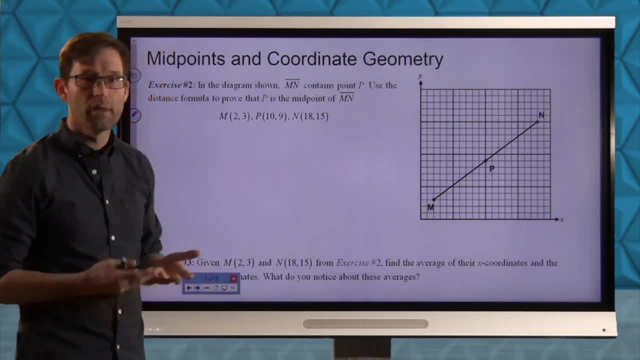 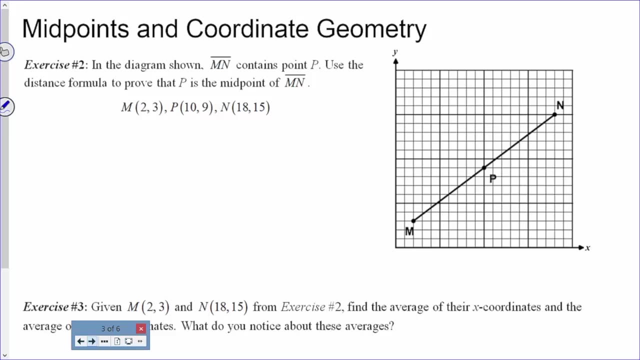 Alright, Here we go. Midpoints and coordinate geometry. Midpoints and coordinate geometry. Exercise two: In the diagram shown, m? n contains point p. Use the distance formula to prove that p is the midpoint of m? n. So I want to prove that p is the midpoint of segment m n. 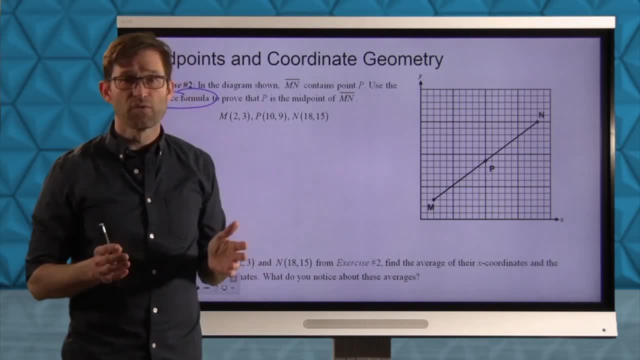 by using the distance formula. Now we learned about the distance formula actually in the last lesson. Hopefully you've already learned it. If you haven't, then this one is gonna be a little bit of a struggle for you. just this first exercise. 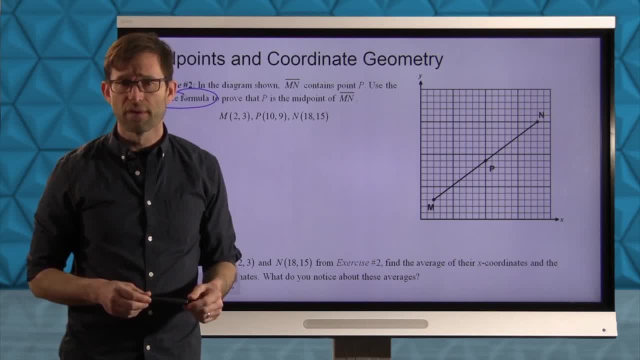 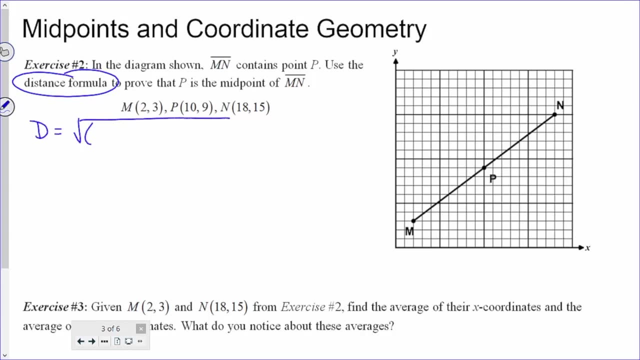 You could probably get away in later exercises without knowing the distance formula, but let me write that down for you. Right, The distance formula is the square root of x two minus minus x one squared, plus y two comma minus y one squared. So if you think about it, 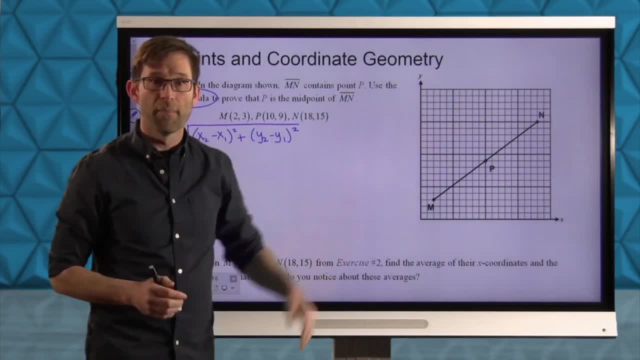 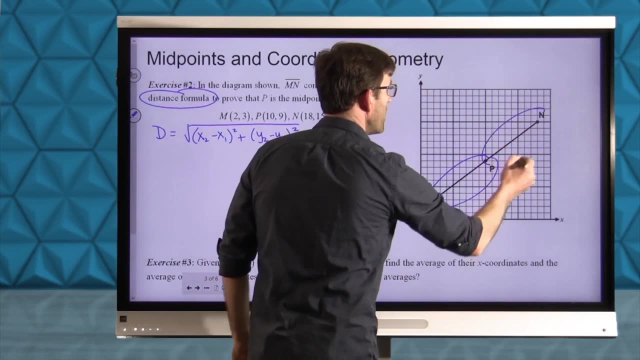 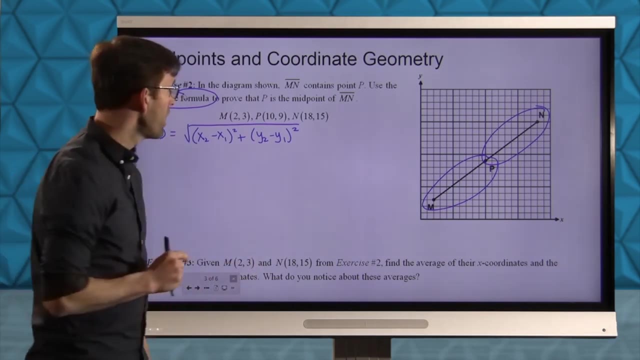 the way that we can prove that p is the midpoint of m? n is by showing that the length of m p right is equal to the length of p? n. Why don't we do m p together, and then you can do p? n on your own? 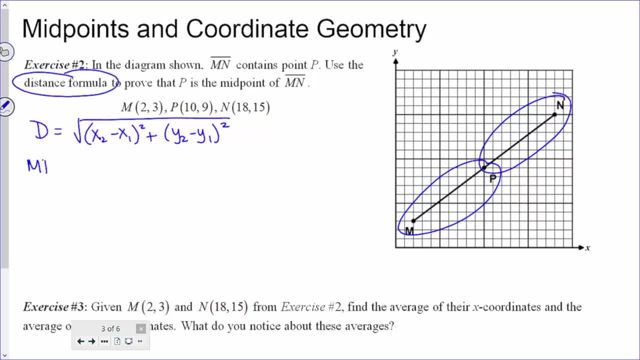 All right. So let's do m p All right. Its length, or the distance between m and p, will be given by 10 minus two, that's the change in x squared plus nine minus three, that's the change in y squared. 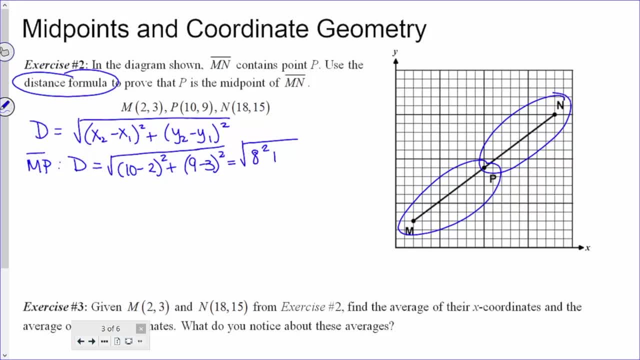 All right, 10 minus two is eight squared. Nine minus three is six squared. We'll get the square root of 64.. Plus 36,, that gives me the square root of 100,, which is 10.. All right. 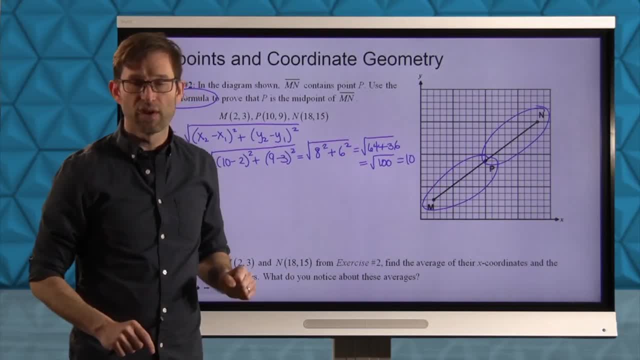 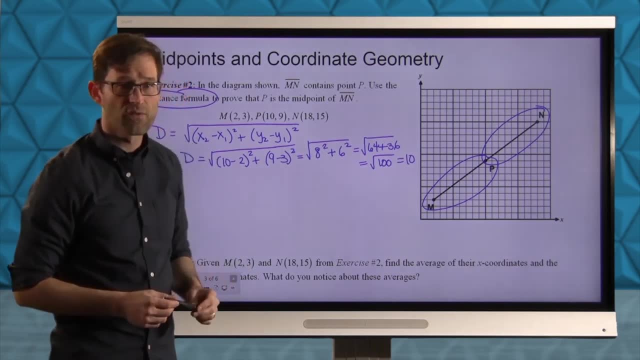 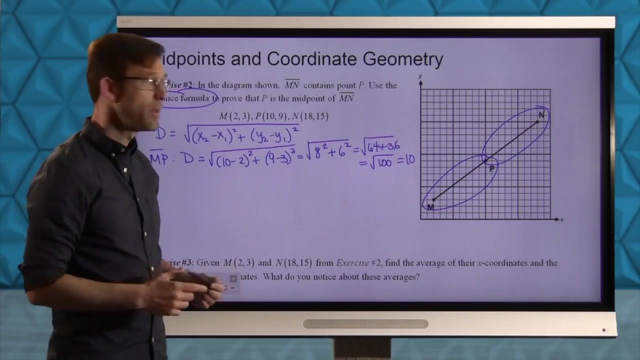 So m, p, m, p has a length of 10 units. Now go ahead and figure out, calculate the length of p n using that distance formula. Take a few minutes for that, All right, let's go through it, All right. 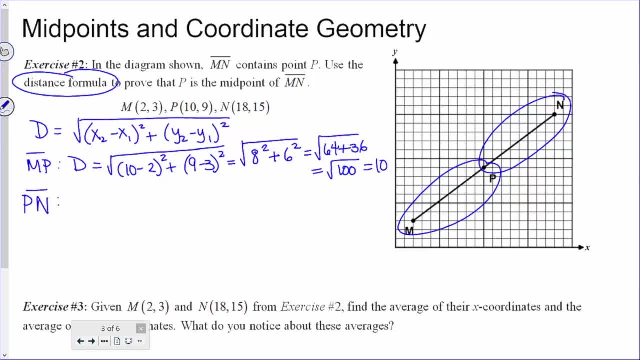 So m p, m p is the length of p n. Okay, I'm going to use these two points now. The distance will be 18 minus 10, squared, plus 15 minus nine squared. All right, 18 minus 10, again is eight. 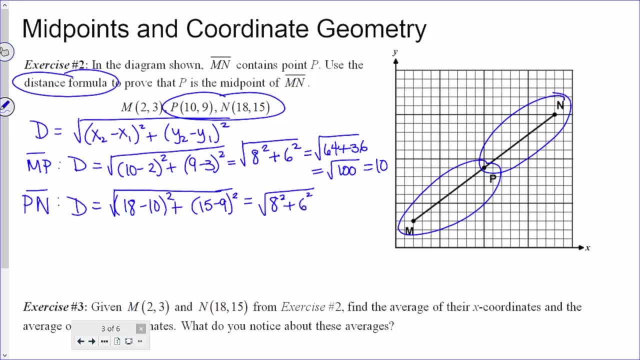 So we get eight squared. 15 minus nine is six again squared. All right, So we're going to add those two together and we'll get the square root of 100, which is also 10.. Right, and that really, truly does prove. 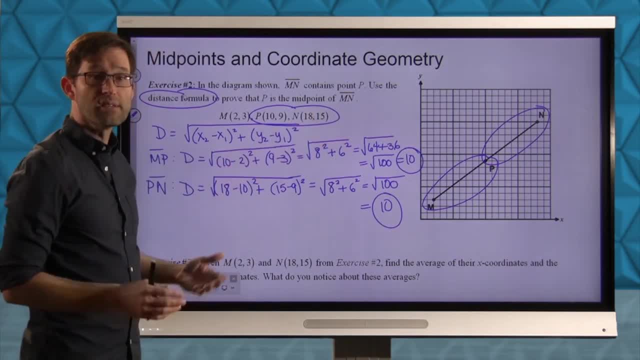 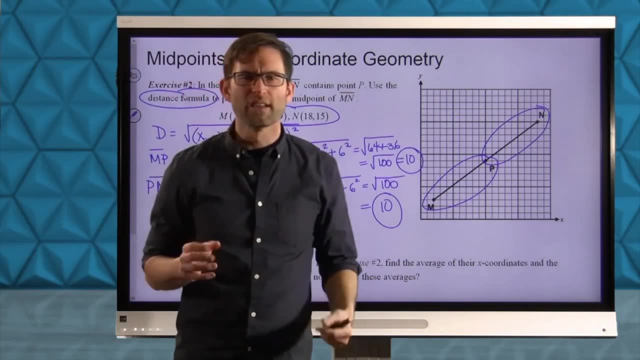 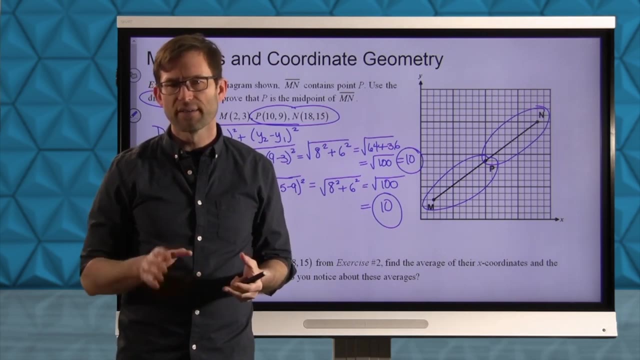 that p is the midpoint of mn because it divides it into two segments that have the same length. One of the things that students tend to like about coordinate geometry is that there are numbers that you can really grasp onto and see right. This is in a huge contrast to the Euclidean proof. 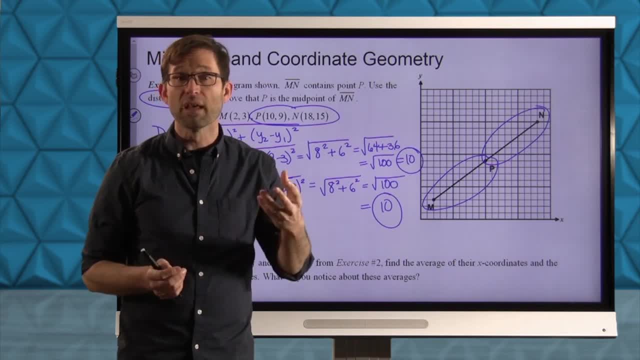 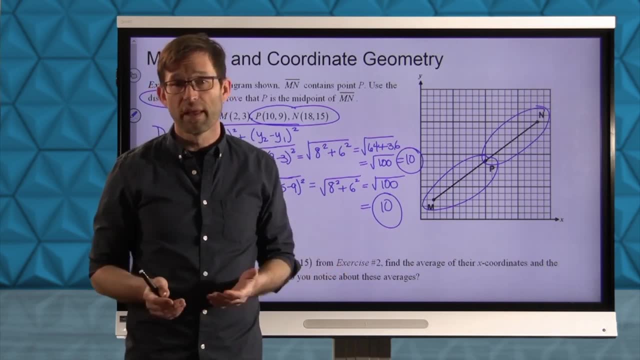 we've done a lot of so far, where it's more just being told: hey, this side is congruent to that side, which means that they would have the same length. but maybe you never know what those lengths are Here. very solid. the length of segment MP is 10 units. the 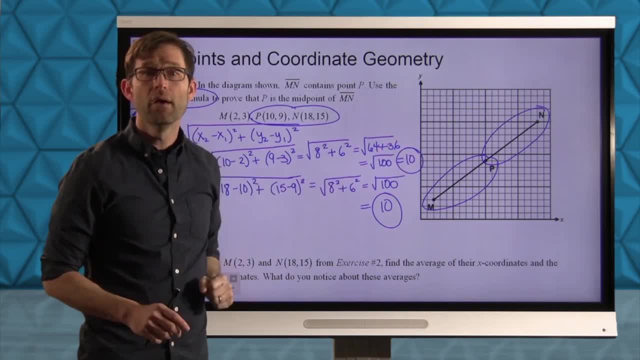 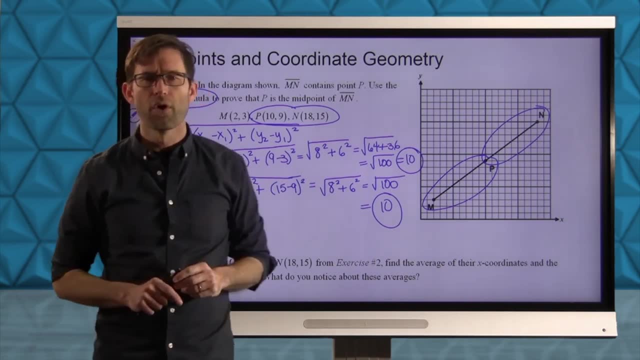 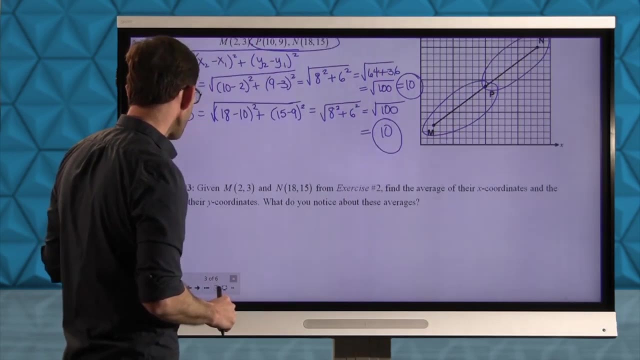 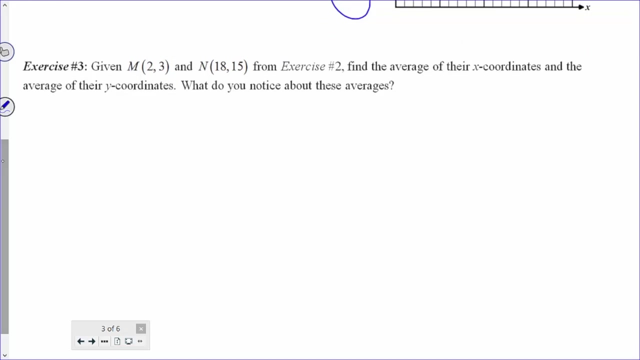 length of segment PN is 10 units and therefore P must lie at the midpoint of that line segment. Now let's try to figure out, though without the distance formula, how we can come up with that midpoint. This goes into exercise number 3.. Exercise 3 says: given M, 2,, 3, and M, 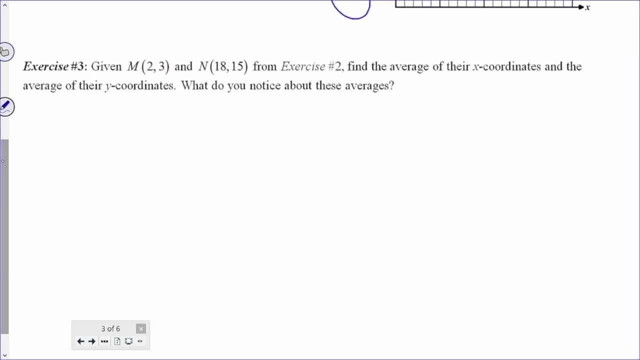 18, 15, from exercise number 2, find the average of their X coordinates and the average of their Y coordinates. What do you know? What do you notice about these averages? Well, I certainly hope you know how to find the. 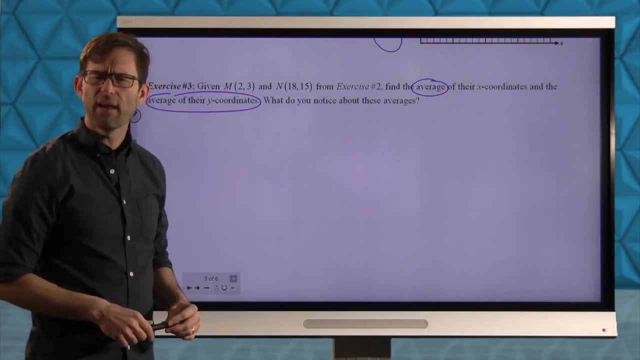 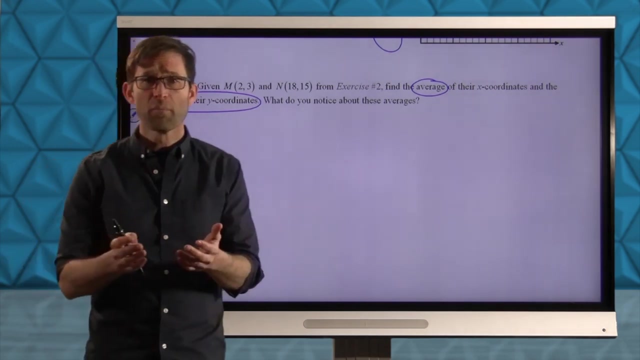 average of two numbers. so go ahead and then see if there's something that's kind of obvious about those two numbers you come up with, All right. Well, to find any average, you add up all the numbers involved and divide by how many there are. Well, there's just. 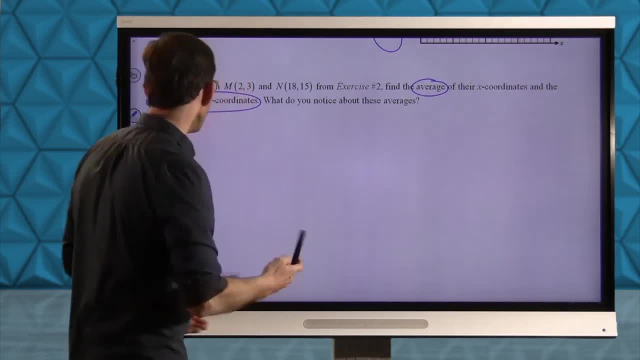 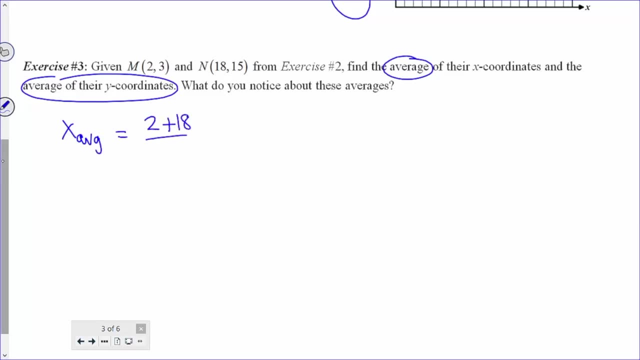 two numbers. We just add those two numbers up and divide by 2.. So, for instance, the average X coordinate would be 2 plus 18 divided by 2, and that's going to be 20 divided by 2, and that's. 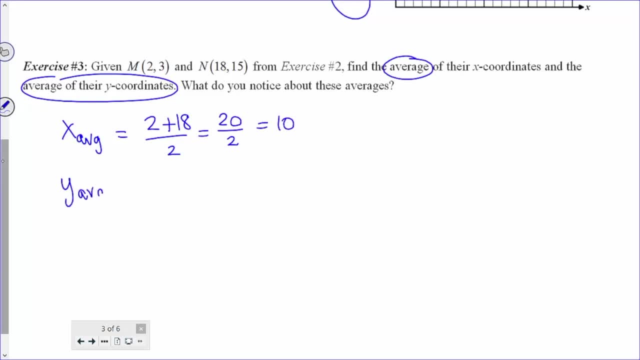 10.. All right, Whatever, The Y coordinate average would be 3 plus 15 divided by 2, and that's 18 divided by 2, and that's 9.. So really you can think of that as being the point 10, 9.. 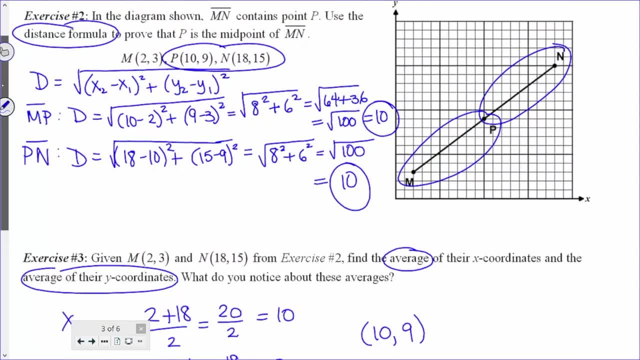 And do you notice that the average X coordinate would be 2 plus 18 divided by 2, and that's 9.. And do you notice anything about the point 10, 9?? Well, let's do it in red, so that it's a lot. 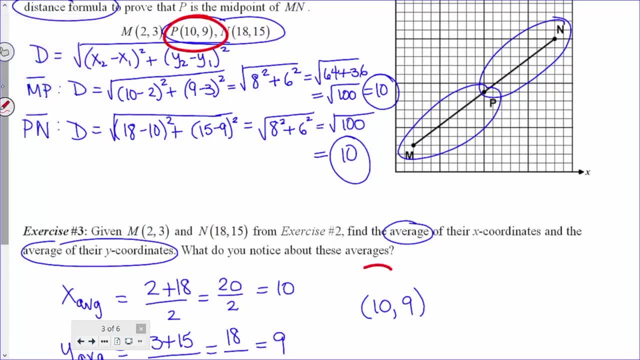 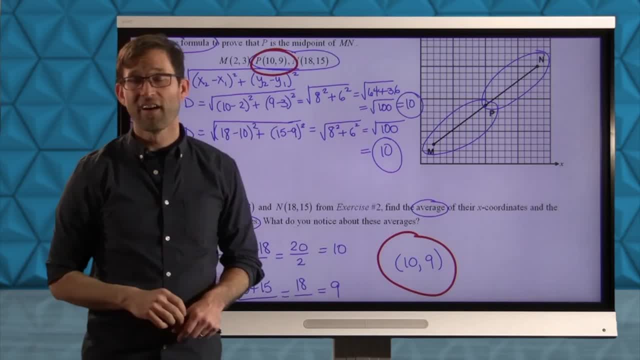 more obvious: 10,, 9 is in fact the midpoint. So how do you find the midpoint of any line segment? You average the X coordinates and you average the Y coordinates, And that should make sense. Generally speaking, averages are a little bit hard to get a feeling for. They're very easy. 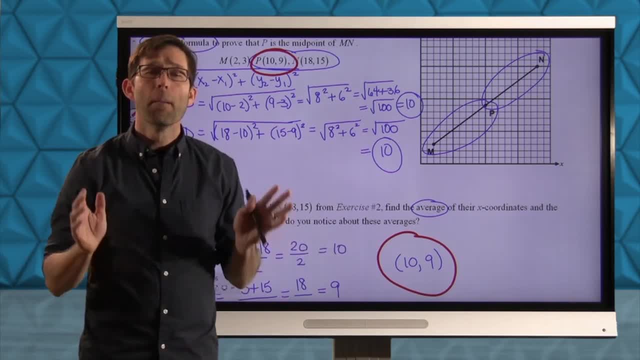 to calculate. They're very easy to calculate. They're very easy to calculate. They're very simple to calculate. Add up all the numbers, divide by how many there are. But when you have two numbers, just two numbers, and you average them. Look, I got average 5 and 7.. 5 plus 7 is 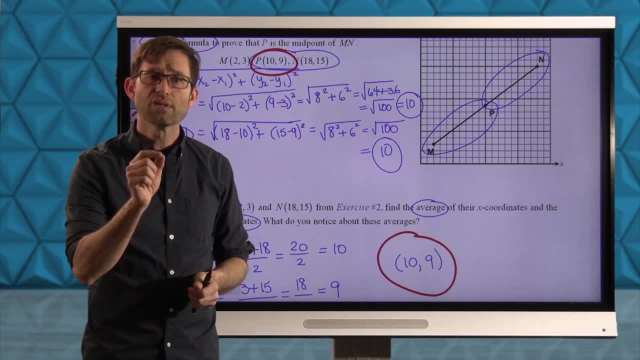 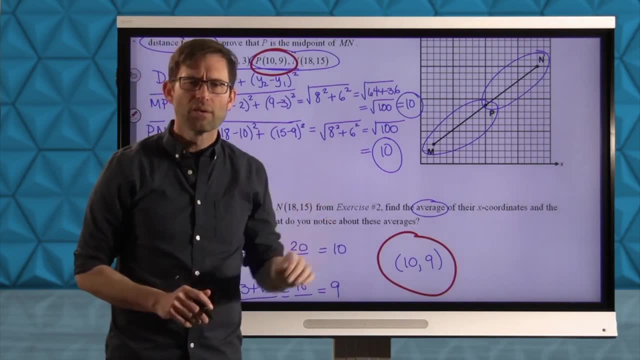 12 divided by 2, and I get 6.. The average is the number that sits right in the middle of the two, And therefore it makes a lot of sense in terms of the midpoint. So let's kind of summarize this. 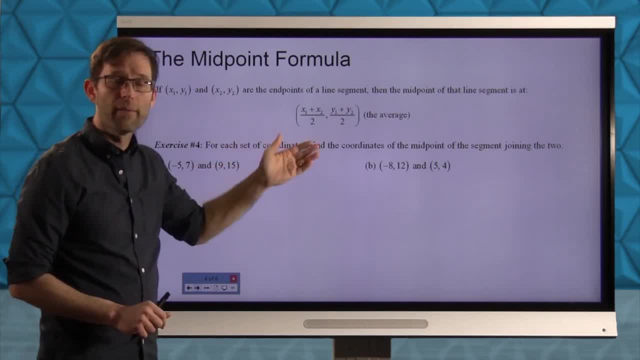 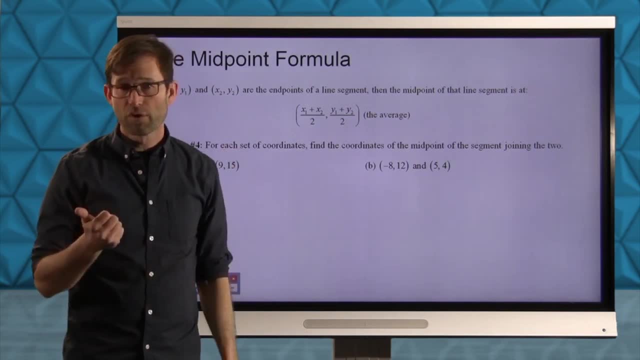 in the next slide with the midpoint formula. All right, Now the midpoint formula really rounds out the figure of the X coordinate. So let's look at the X coordinate. So let's look at the X coordinate. There are three extremely important formulas of coordinate geometry, The first being the slope. 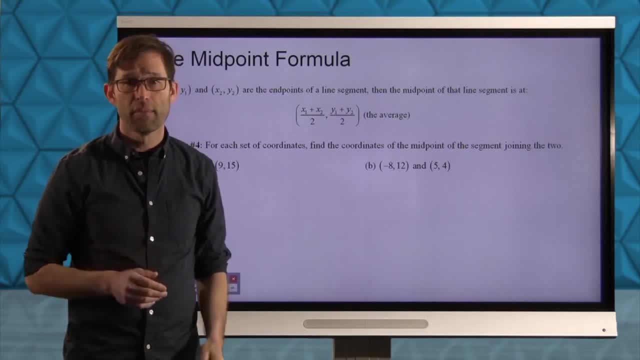 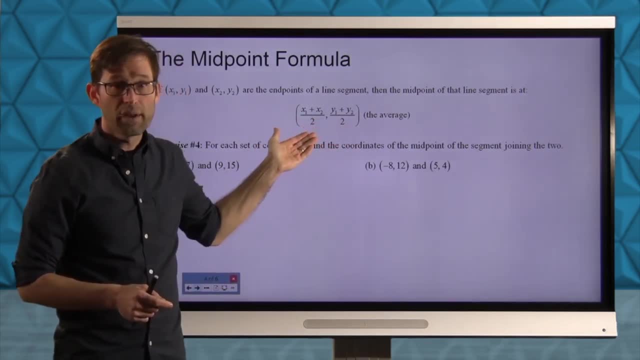 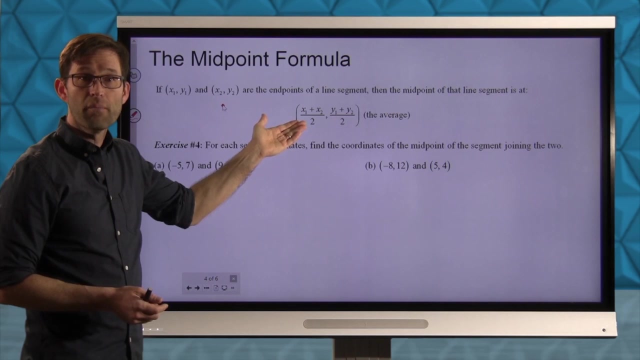 formula, the second being the distance formula and now the midpoint formula. The midpoint formula, no great surprise, comes in the form of a coordinate point. But here's the key, right. If you've got a line segment that's got endpoints at X1, Y1, and X2, Y2, then to find the midpoint. 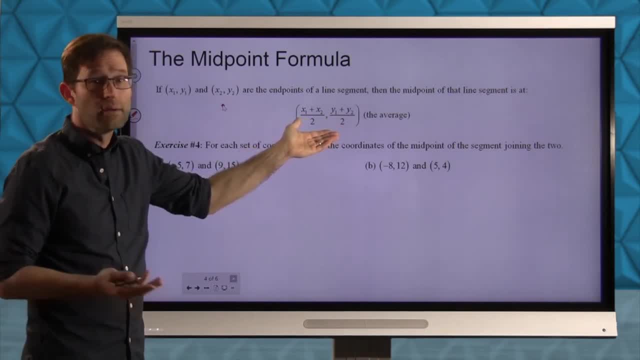 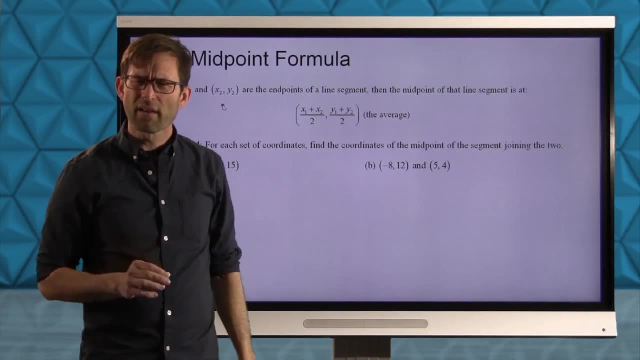 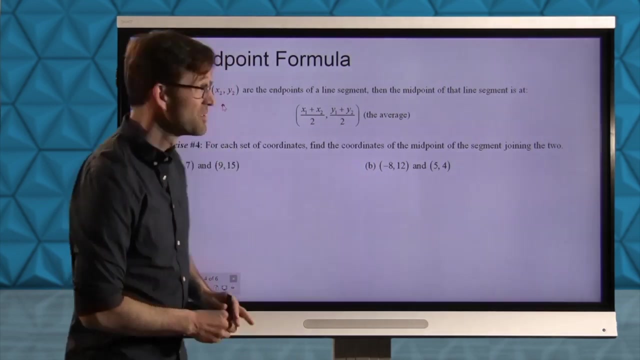 all you have to do is average the X and average the Y. That's it. It is the easiest, in my personal opinion, of the three formulas to use. Ironically, it seems to be the one that students struggle the most with, And yet, average X, average Y and you've got the midpoint. So let's get a little. 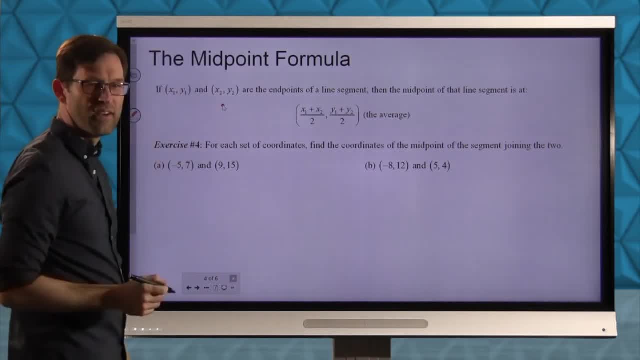 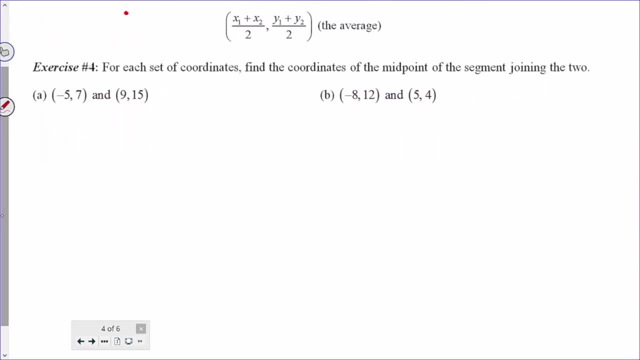 practice with that. No square roots involved, Nothing really particularly messy, All right. Exercise number four says: for each set of coordinates, find the coordinates of the midpoint of the segment. joining the two, Joining the two. All right. So let's say I've got a segment that's got these two endpoints and I want. 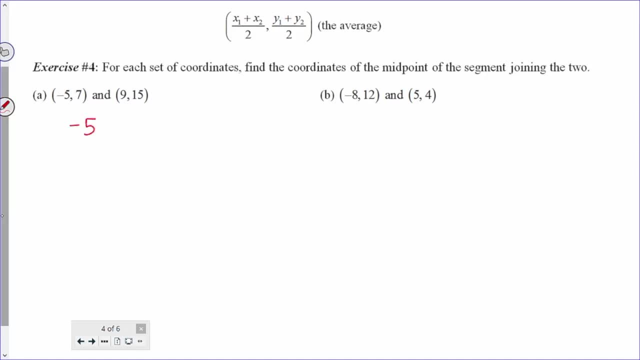 to find the midpoint. So what do I do? Well, I take negative five plus nine, the two X coordinates, and I divide by two. Negative five plus nine is positive, four Positive. four divided by two is two. That's my average X coordinate. My average Y coordinate on: 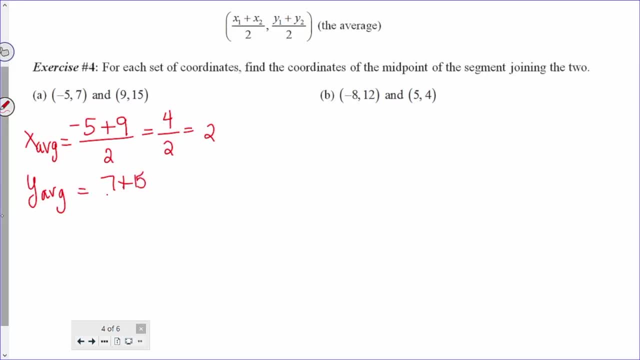 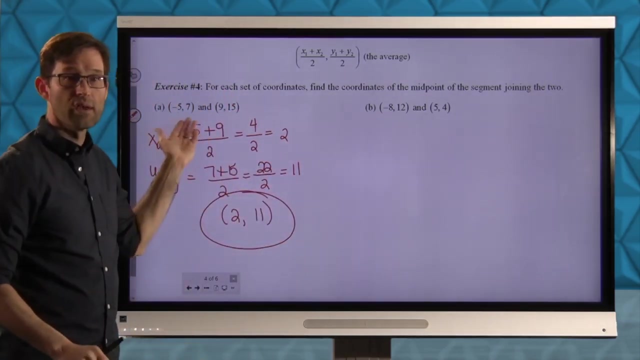 the other hand, would be seven plus fifteen divided by two, which is negative. five plus twenty-two divided by two, and that's eleven. So the midpoint on a line segment that has these two coordinates as its endpoints is two comma eleven. They don't get much easier. 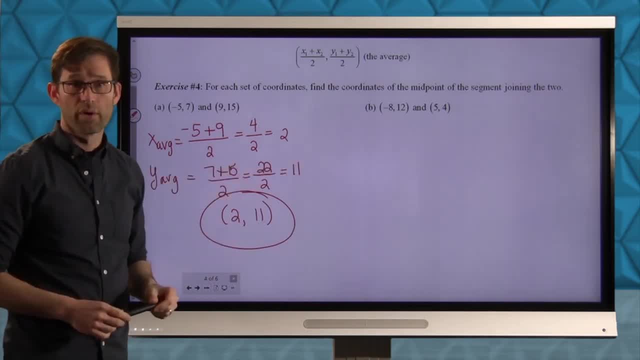 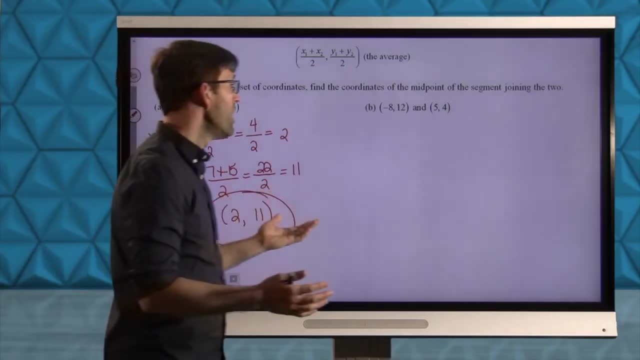 than that. Why don't you go ahead and do it for those two coordinate points? All right, Let's go through it. You can kind of lay it out as X average, Y coordinate to Y average, or you could do it all within sort of the parentheses, like this: 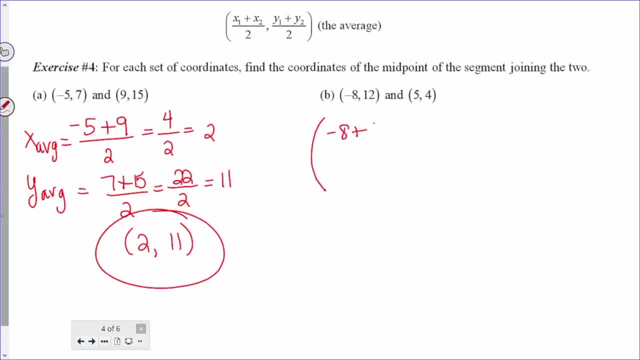 So I could do something like this. I could say: well, I have negative 8 plus 5 divided by 2, comma: 12 plus 4 divided by 2, right, That will give me negative 3 divided by 2 and 16 divided by 2.. 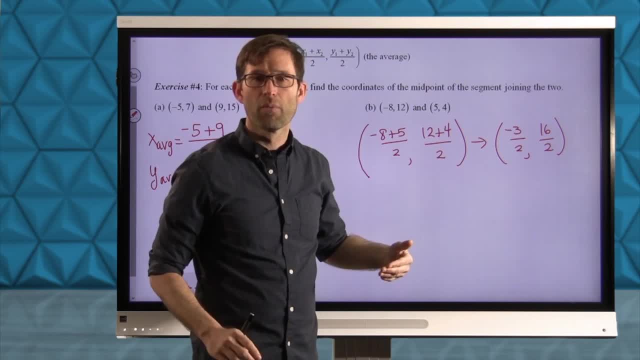 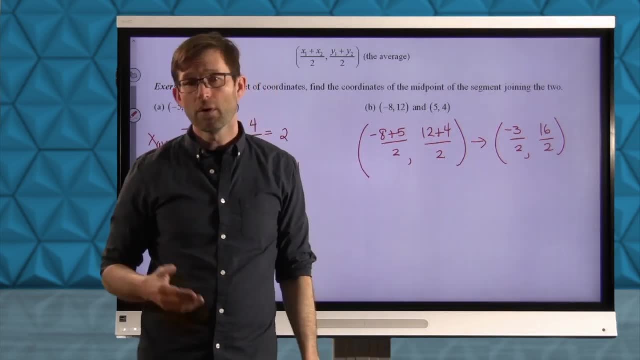 Now, of course, negative 3 is not nicely divisible by 2.. So what should you do? Well, you could leave it as negative 3 halves, that would be fine. You could write it as negative 1 and a half, or you could even do negative 1.5, alright. 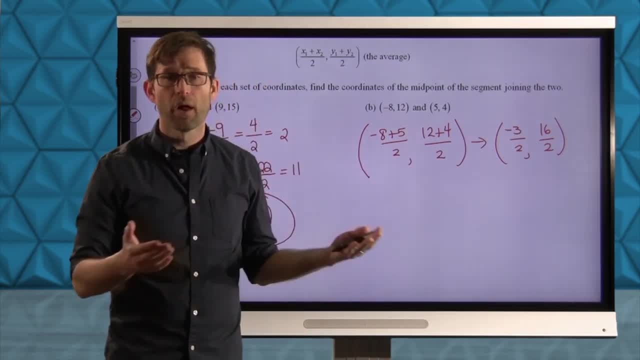 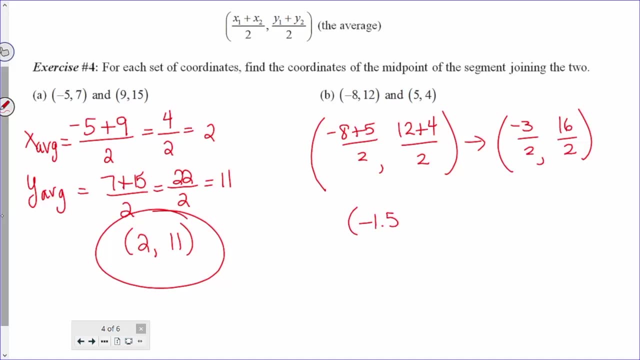 If your teacher has a preferred way for you to leave an answer like that, I would follow what your teacher says. I personally don't have any problems with decimals. I kind of like them. so I think I would probably say negative 1.5 and 8.. 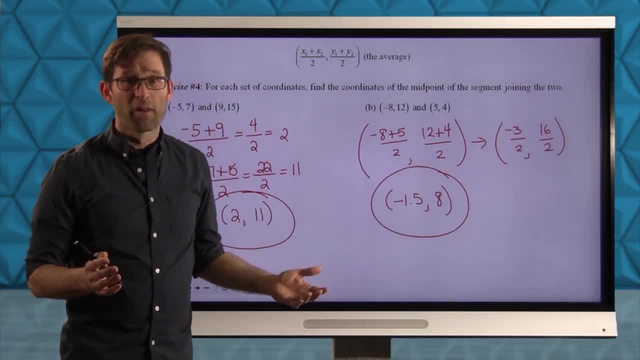 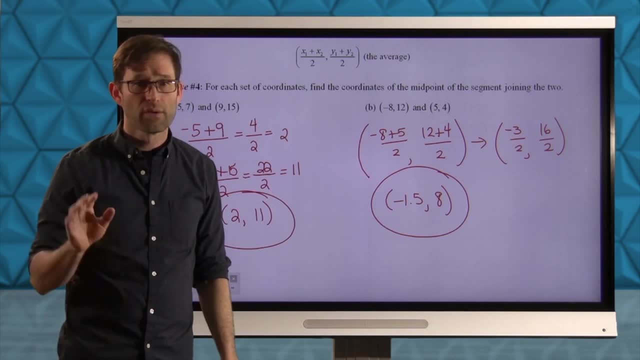 Negative: 1.5 and 8. The midpoint formula- What more is there to say? The distance formula is kind of challenging. subtract, subtract, square, square add. take the square root, possibly simplify radicals, all that kind of business. 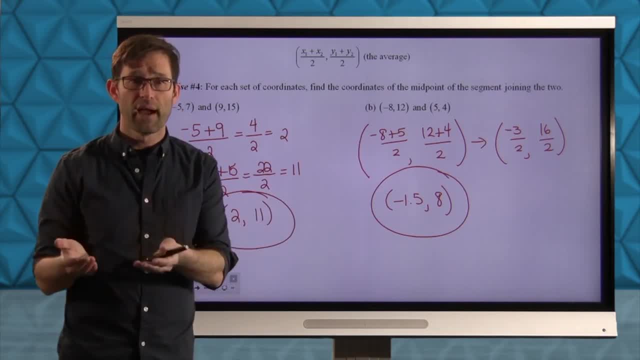 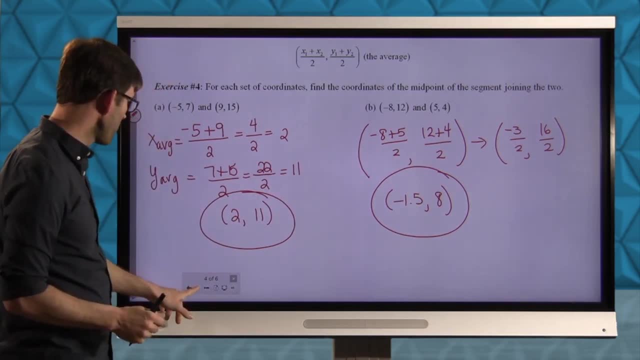 The midpoint formula. find the average of the x coordinates, find the average of the y coordinates, and you have the midpoint. It's pretty nice. Okay, let's get a little more work with this. Not much, though, because there's not much to say, right. 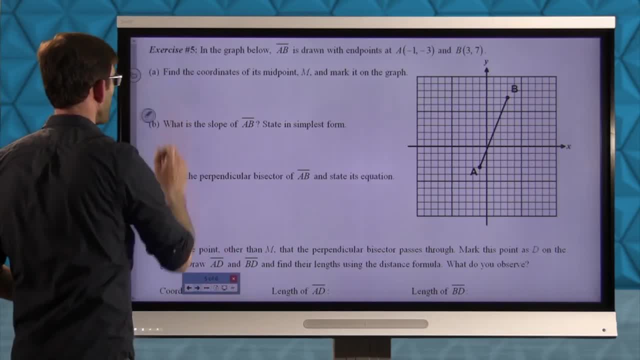 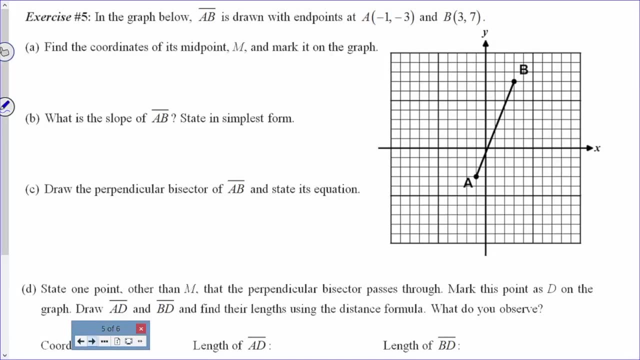 Let me change back to blue real quick. Let's take a look at about the most challenging problem we're going to do today, exercise number 5.. In the graph below, AB is drawn with endpoints at, and Letter A asks us to find the coordinates of the midpoint of M and mark it on the graph. 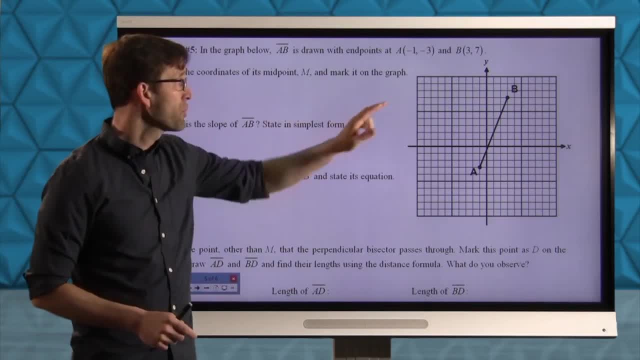 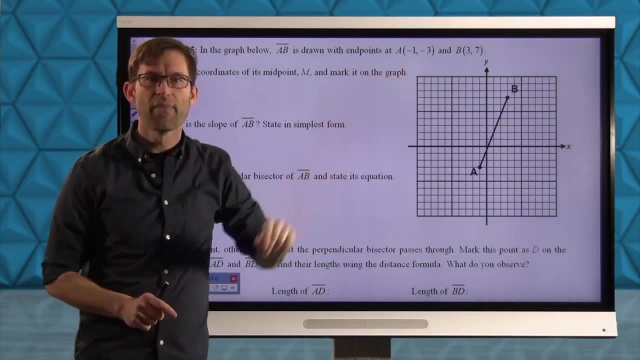 Great Alright. so why don't you go ahead and do that procedure? just use the formula. trust me. use the formula and come up with the midpoint based on those two coordinate points and then plot it. Then we'll revisit the problem. 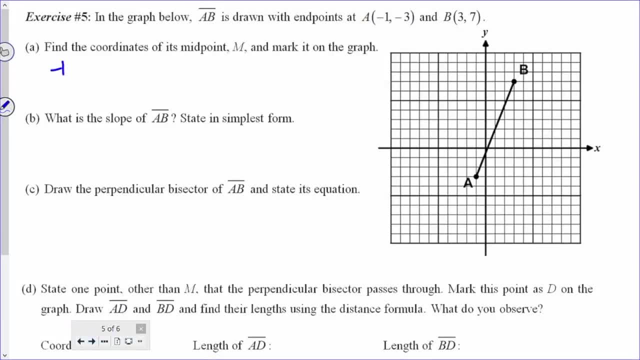 Alright, let's go through it Again. pretty easy. Take the x coordinates: negative. 1 plus 3 divided by 2 equals positive. 2 divided by 2 equals 1.. That's my x coordinate. My y coordinates will be negative. 3 plus 7 divided by 2 will give me 4 divided by 2 will 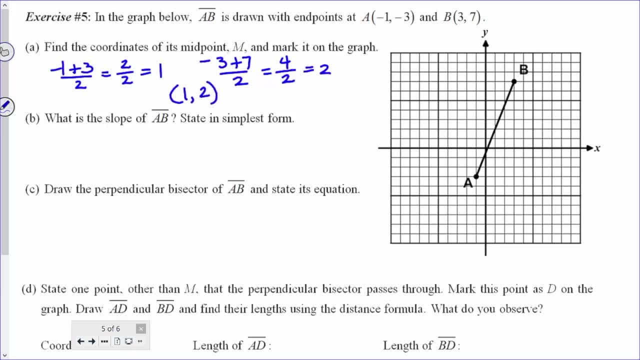 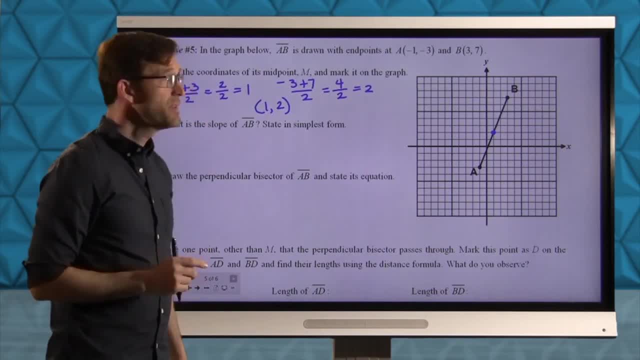 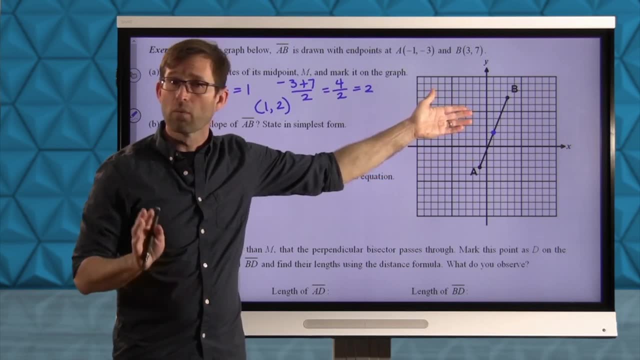 give me 2.. So the midpoint looks like it's got coordinates at And that's right there. Alright, one of the nice things is that visually speaking, it looks right, and also, of course, if we got a point that didn't even lie on that line segment, we would definitely know. 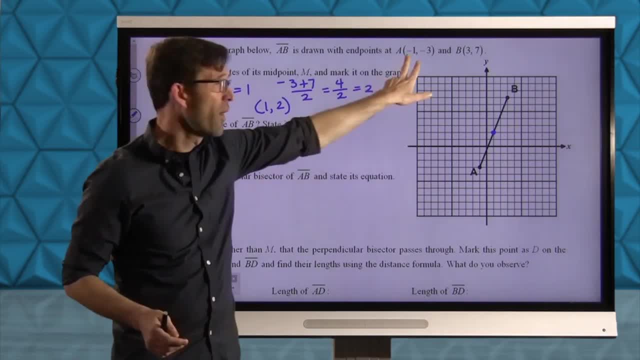 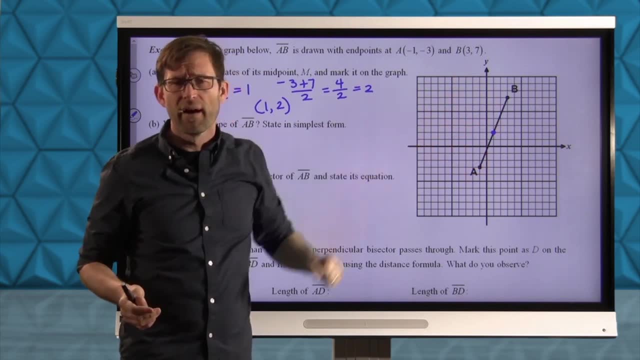 that it was wrong. So if I had done something weird like I don't know, average these two and then average those two somehow, I don't know, you know, we would get a point that wouldn't even likely lie on the line segment. 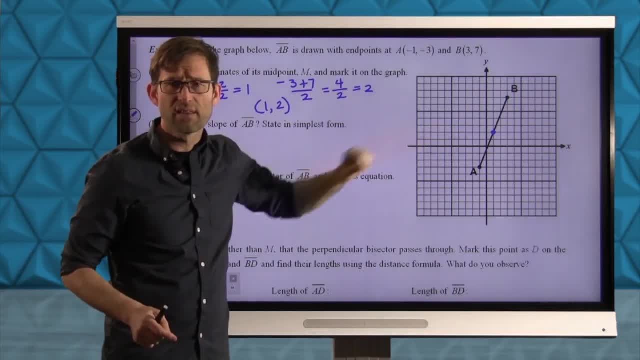 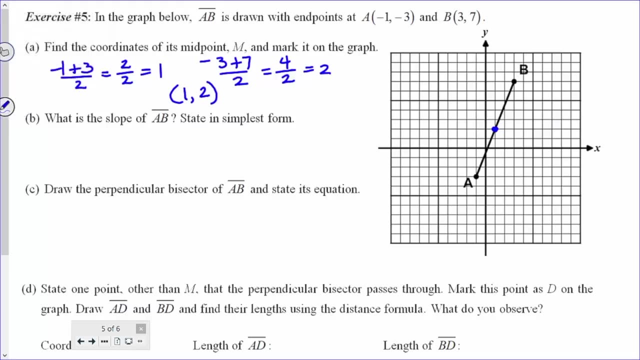 So that at least we know lies on the line segment and it definitely looks like it's at the midpoint. Alright, let's take a look at letter B. Letter B says what is the slope of state in the simplest form. So I just want to know the slope of. 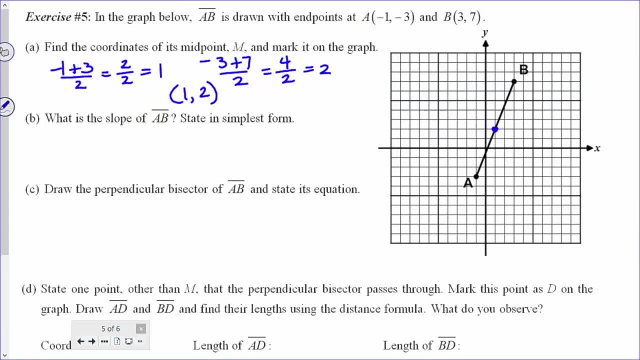 Why don't you go ahead and do that? Alright, let's do it Now. I'm going to be kind of formula driven here. We could do it graphically, but I'm going to try to review every one of the major coordinate geometry formulas in this lesson. 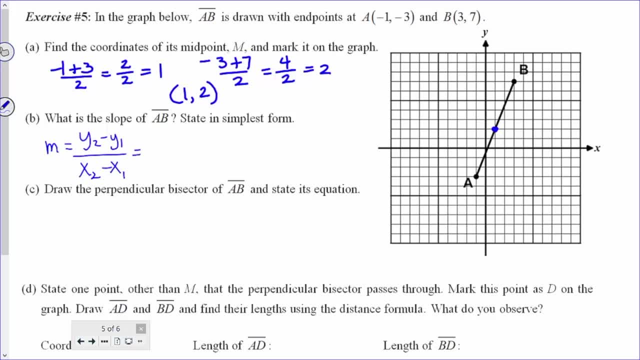 So the slope formula divided by That will be 7 minus 1.. Alright, 7 minus negative 3, all divided by 3 minus negative 1, gives me 10 in the numerator, 4 in the denominator. I can reduce both of those by dividing both by 2 and I get a slope of 5 halves. 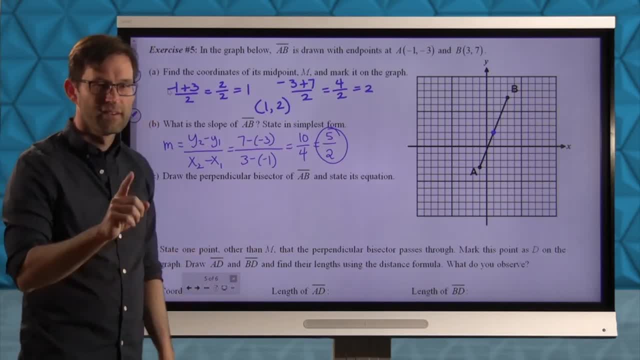 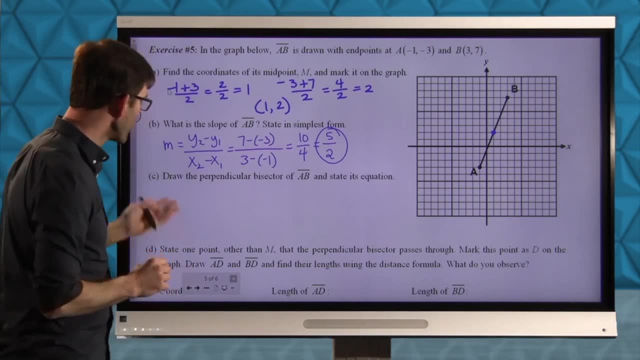 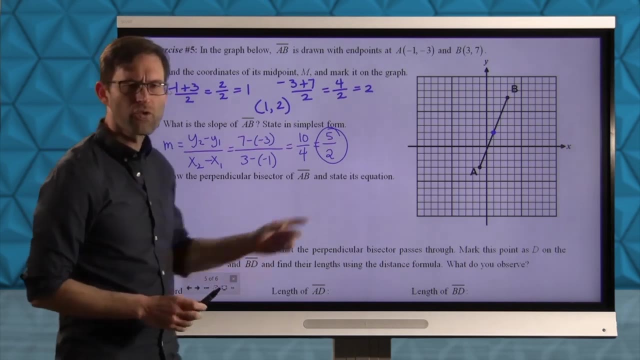 Alright. so the slope of AB is 5 halves. Now letter C: Draw the perpendicular bisector of AB. draw the perpendicular bisector of AB and state it. State it's equation. So now I want to draw the line that bisects AB, so it's got to pass through the midpoint. 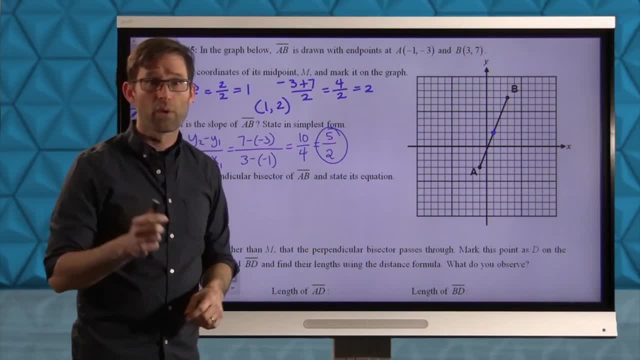 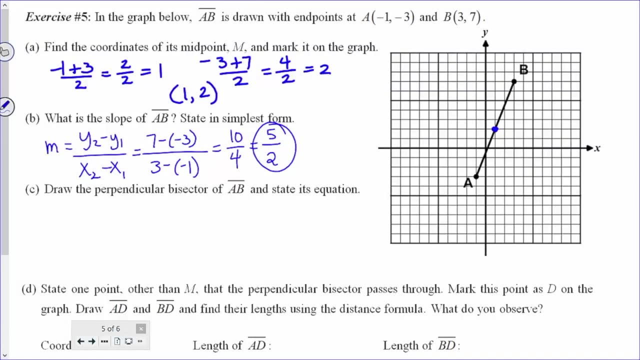 and is perpendicular to it. Do you know, do you remember, what the relationship is between the slope of AB and the slope of that line that's perpendicular to AB? Ah Well, the perpendicular line will have a slope that is the negative reciprocal of AB. 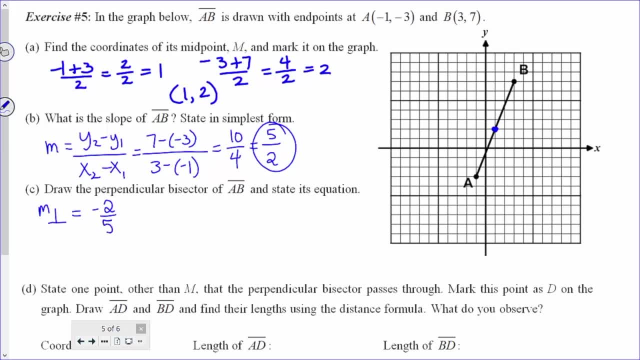 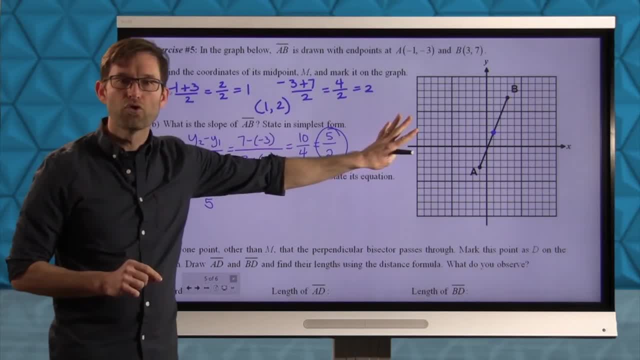 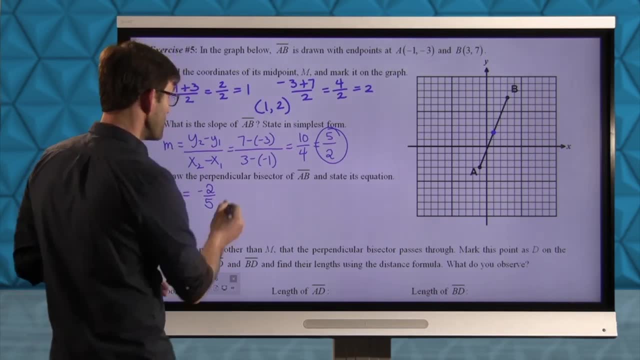 Alright, Let's do it, Let's do it. So let's draw a slope of AB, So it will have a slope of negative 2 fifths. See if you can use that slope now to draw the perpendicular bisector And if you can remember how to write its equation. and I would suggest writing its. 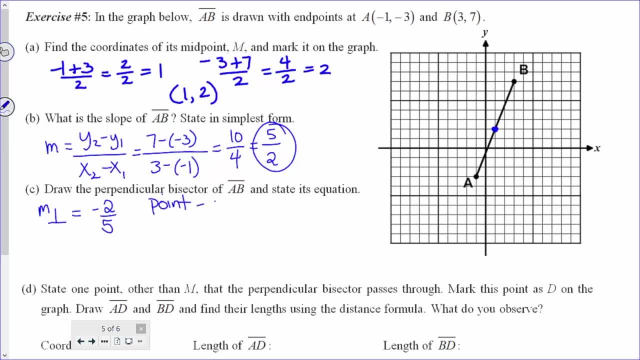 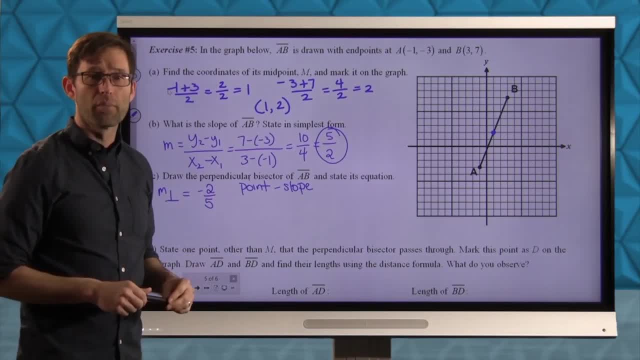 equation in point slope form instead of slope intercept form. well, go ahead and do so, But first draw in the perpendicular bisector. And then we'll go ahead and do that, But first draw in the perpendicular bisector, Alright. 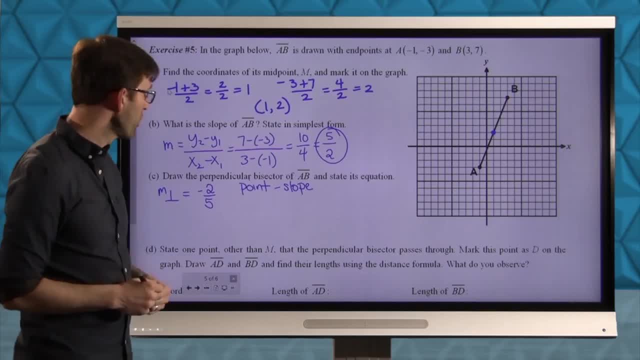 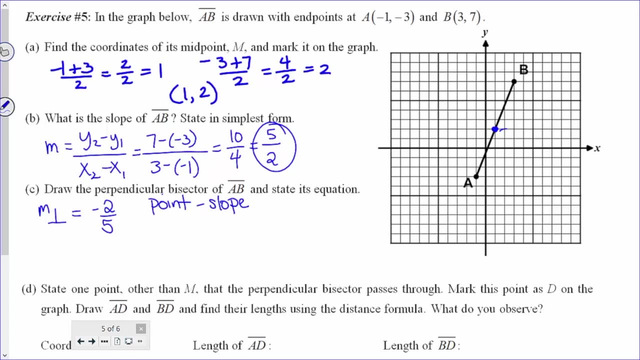 Do you know? do you? can you see? Alright, let's go through it. Well, we know we've got a rise divided by run of negative two-fifths, which means I'm going to go five units to the right and two units down to get my next point, or I can 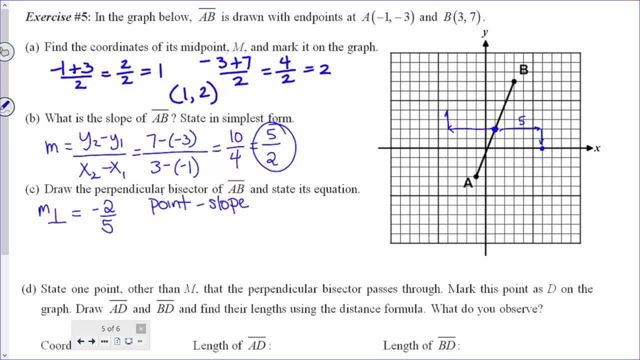 go five units to the left and two units up. I think I'll do one more of those, Alright. so all those points line the perpendicular bisector. is that right? let me just make sure. yep, yep, okay, great. 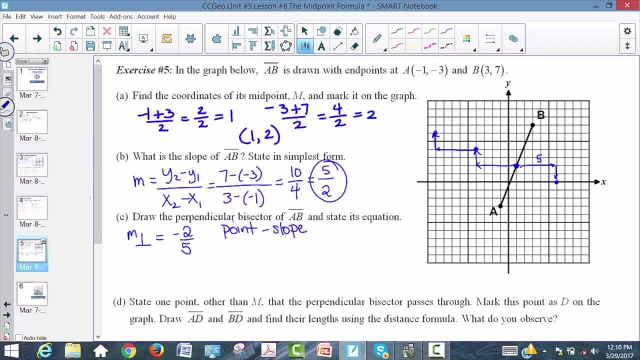 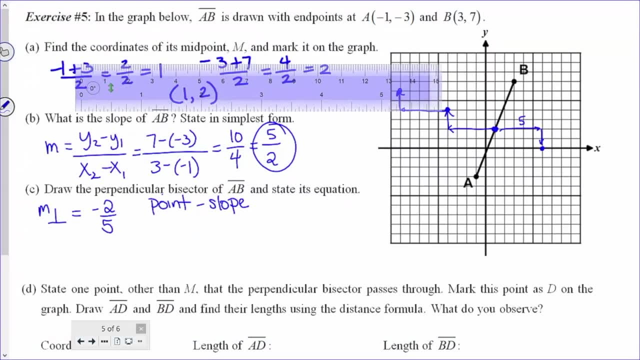 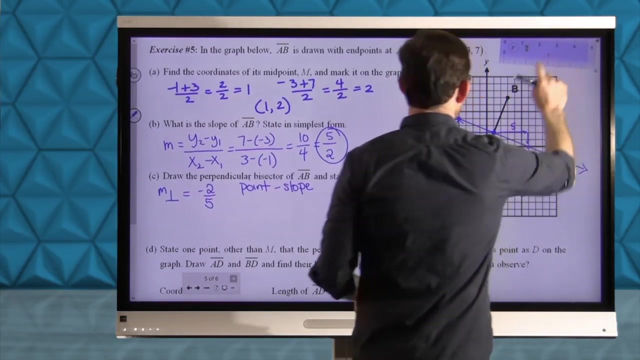 And I don't have a ruler. let me go grab a ruler real quick. Thank you, Go back to full screen And now let me use my ruler. Okay, And draw that perpendicular bisector. Remember not to minimize it, but one thing that is true is that the perpendicular bisector 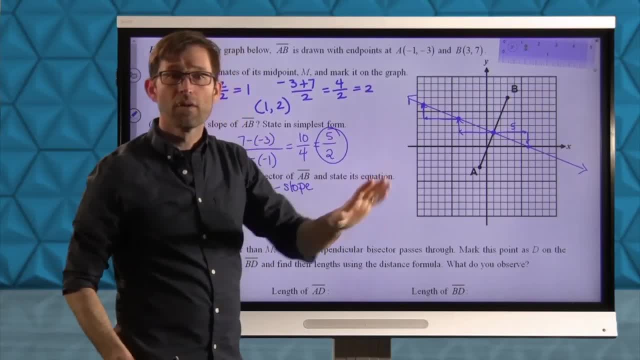 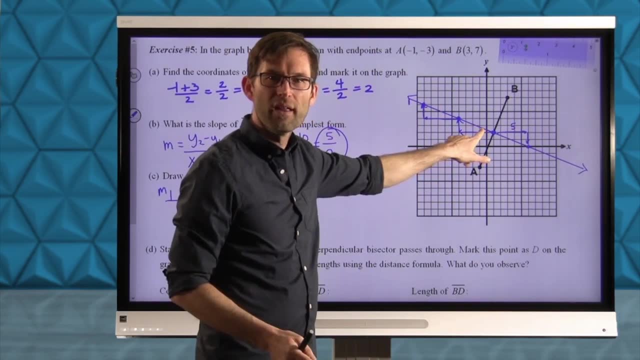 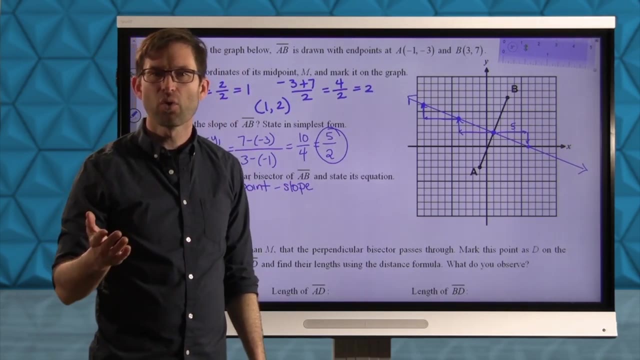 must go through the midpoint. It must. Now let's write its equation. okay, Does it have a nice y intercept? It doesn't particularly right. The y intercept of the perpendicular bisector isn't particularly nice. so using y equals mx plus b, not a great choice. On the other hand, a few lessons ago, we learned about what was. 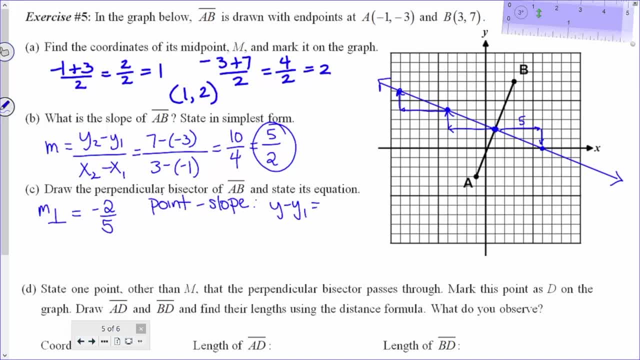 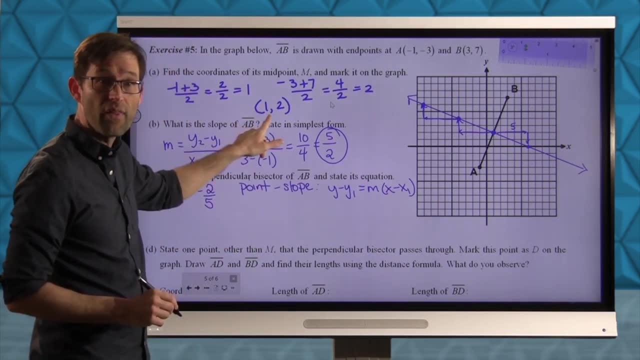 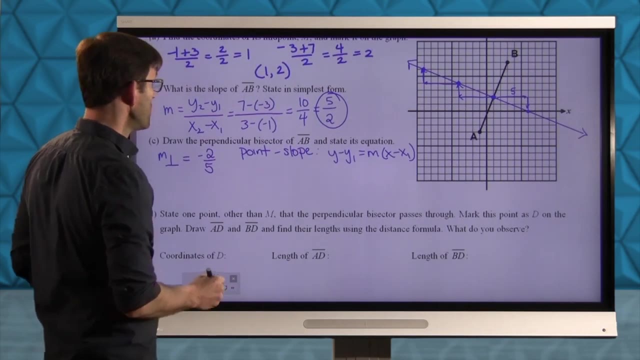 called the point slope form of a line. y minus y1 equals m times x minus x1.. Okay, and the beautiful thing is, we know a very nice point that lies on that perpendicular bisector, specifically the midpoint. We also know its slope negative two-fifths, so we can write the equation by just. 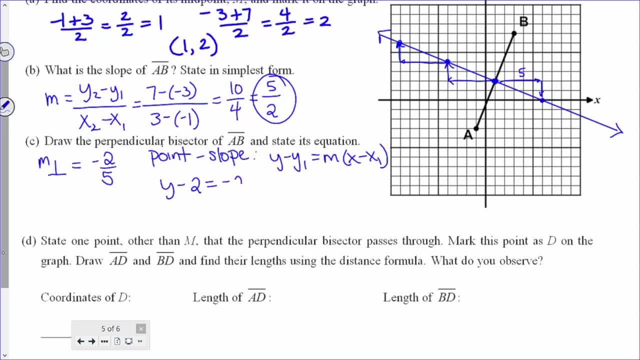 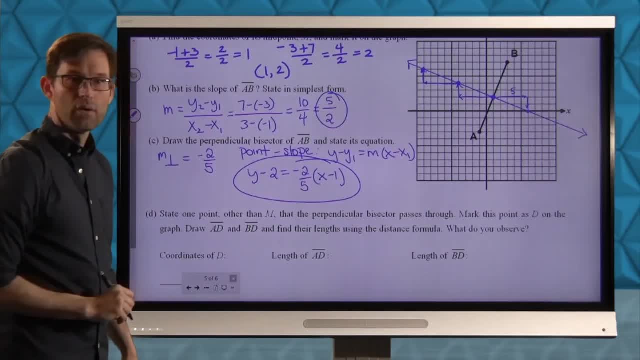 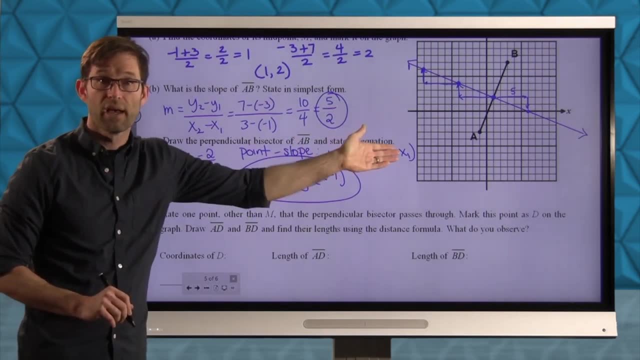 doing this, y minus 2 equals negative two-fifths times x minus 1.. Right and again, all I'm doing is using the point 1, comma 2. in this general form: y minus y1 equals m times x minus x1.. I'm using: 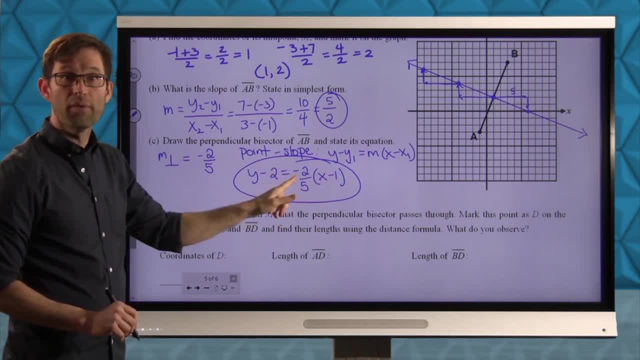 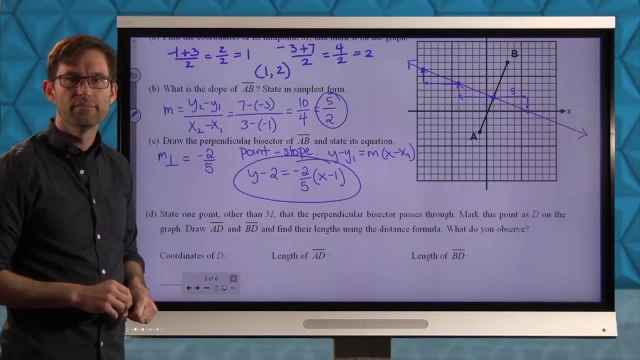 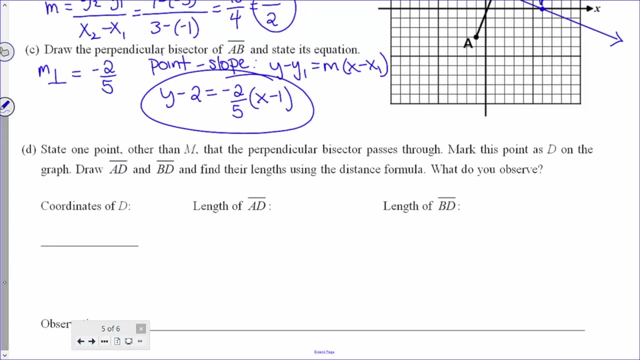 the point 1, comma 2.. And then I'm getting the slope negative two-fifths from that perpendicular relationship. All right, one last little piece, letter d. Letter d says: state one point other than m that the perpendicular bisector passes through. Mark this point as d on the graph. 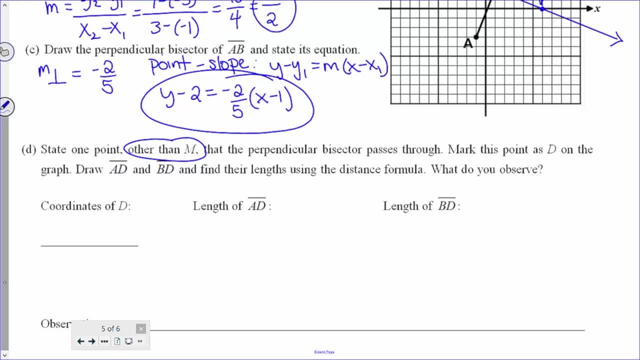 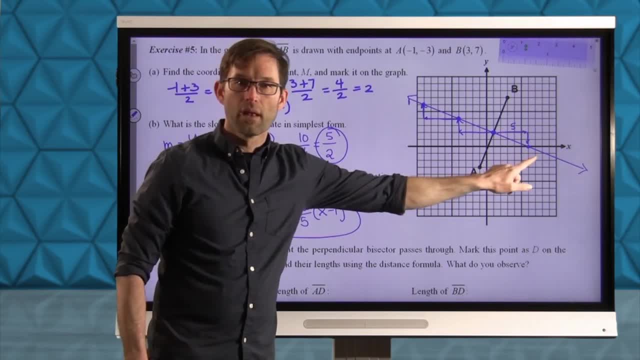 draw ad and bd and find their lengths using the distance formula. What do you observe? Well, there are obviously an infinite number of points that lie along that perpendicular bisector, but there are also some that are nicer than others, Right, for instance, there. 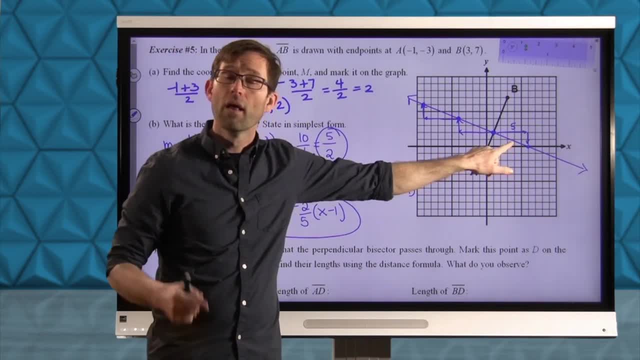 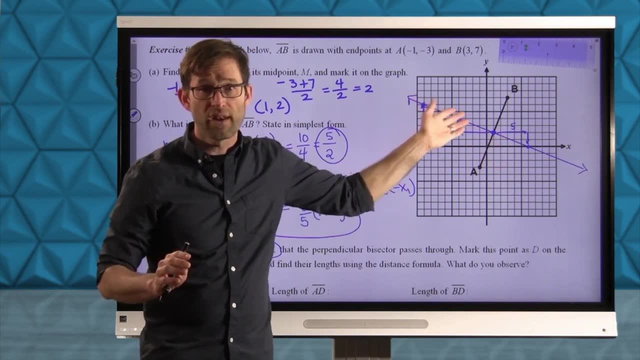 are the three points we marked here, here and here that are particularly nice. Now, this part of the exercise works with any of those three nice points, or even any of the not so nice points. I'm guessing that we want to stick with one that's pretty nice So. let me pick one. Okay, let's find I need to pick a 3 tip points, 3 differences within the Multi/. Then let me take that number over to i. i So I'manterizes point i with that number. All right, I'manderizes point i with that number. i So, And I got just a bit more obvious. 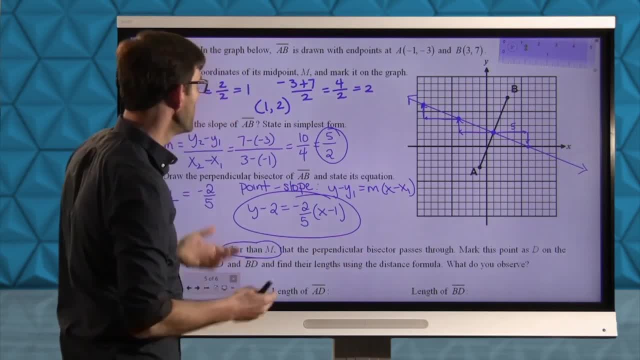 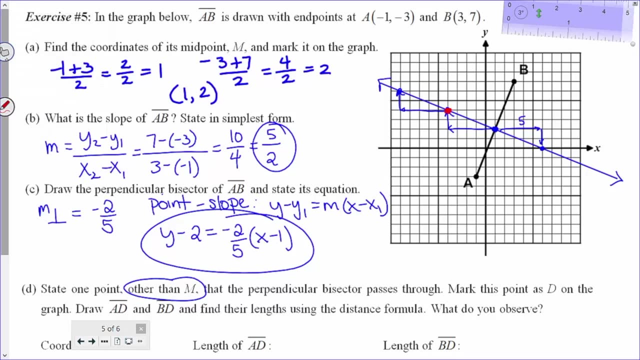 three point points and I have the proper amount of points and that will get better than some pick one. Okay, let me go with one that makes sense. I'm going to go with red here, Alright, and I think I'll just use this. Specifically, I'll use the point negative four comma four. 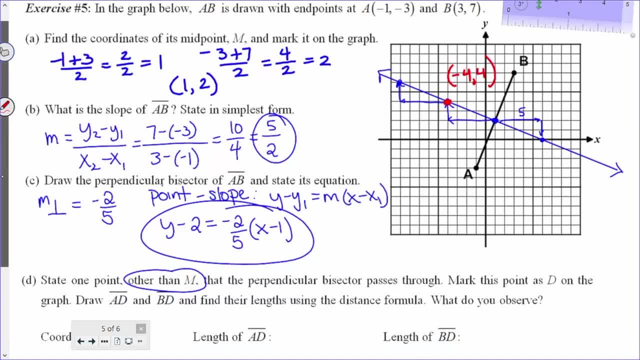 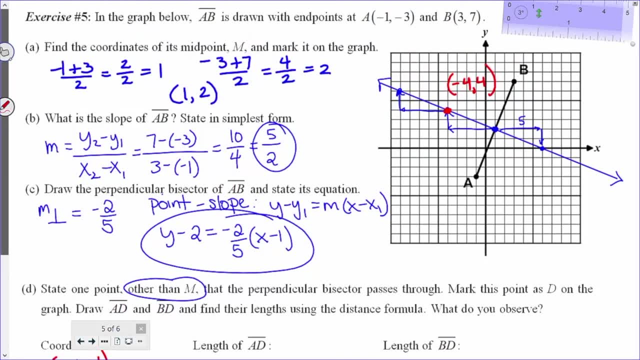 That lies on the perpendicular bisector, So let me just kind of throw that down in here. Four comma four. And then what the problem also asked me to do was draw in AD. I'm going to label this as point D: To draw in AD. come here, come here, come back to me. There we 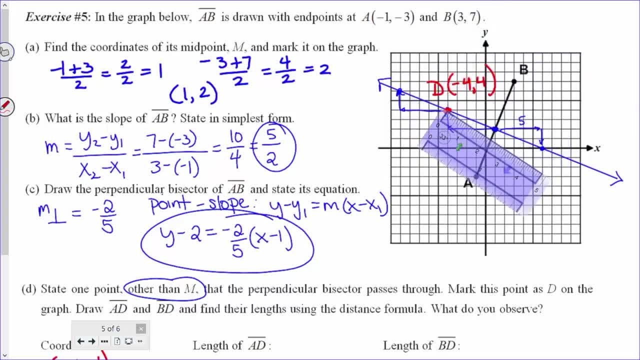 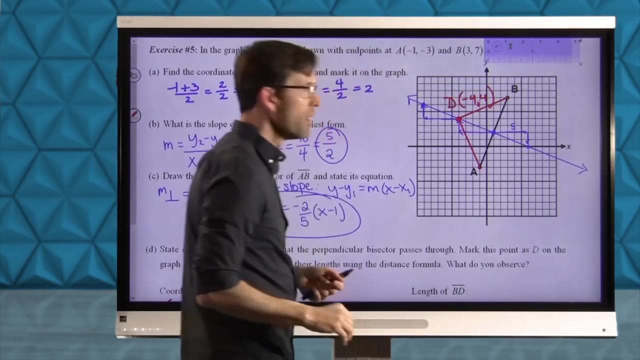 go Draw in AD and BD. I think I'll just stick with it in red to contrast that nice blue that we've got up there. So here's AD And here's BD, BD, And now we'll get rid of our room. Alright, and what I'd like to do now is I'd like to 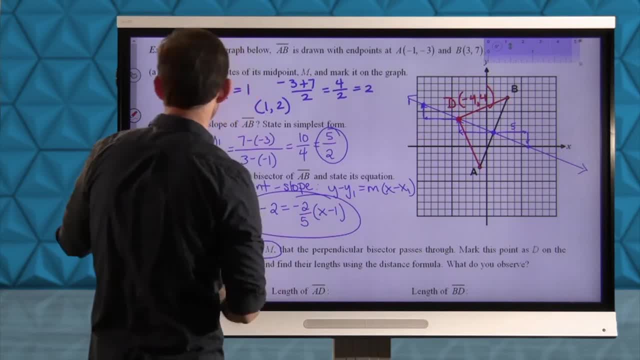 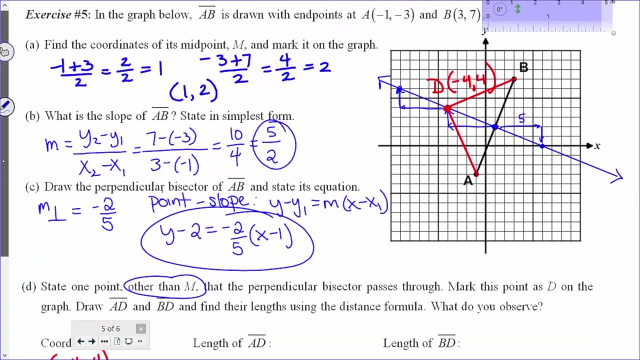 actually calculate the length of AD and length of BD. Okay, real quick, I think. what I'd like to do is write down the coordinates of A and B before we – A is negative one, three and B is negative two. Do you understand? Do you understand? You understand, Or do you? 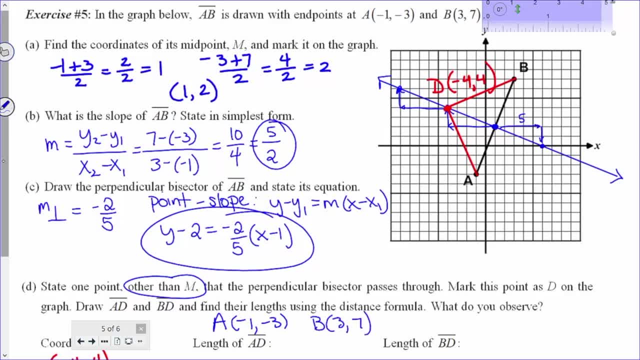 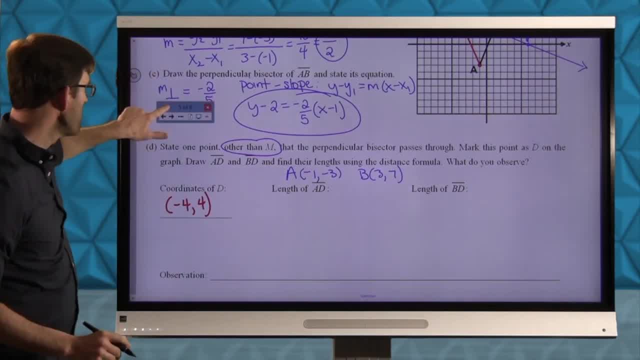 Do you understand? Do you understand Right? Did you understand? Of course you did. Okay, B is 3, 7.. And now let's figure out the length of AD and the length of BD and make an observation about it. 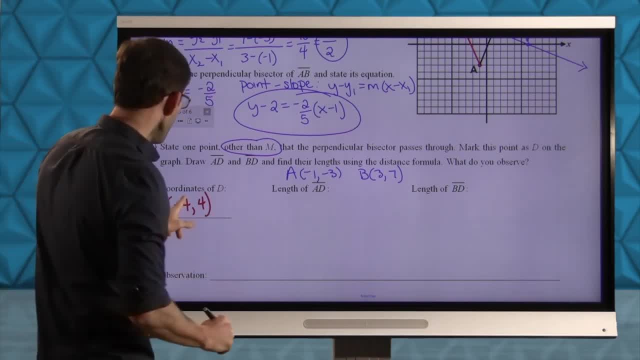 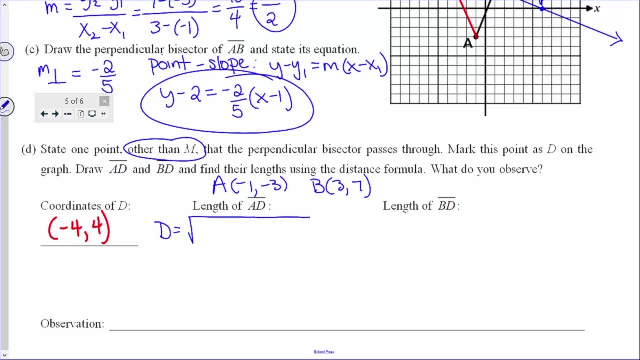 Okay, Let's do AD together and then you can do BD. So here's A, here's D and here's A. Let's do the distance formula. All right, Let's square root of negative 1 minus negative 4 squared. 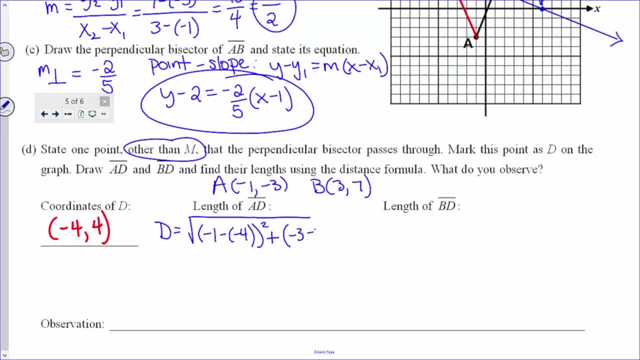 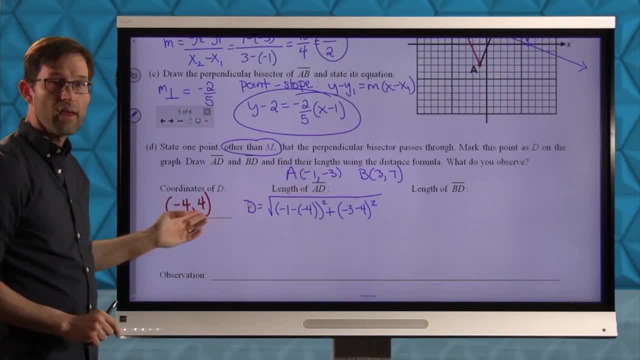 Plus negative 3 minus 4 squared. All right Again, all I'm doing is using the distance formula with point A and point D: Negative 1 minus negative 4 squared. negative 3 minus 4 squared. That's it. 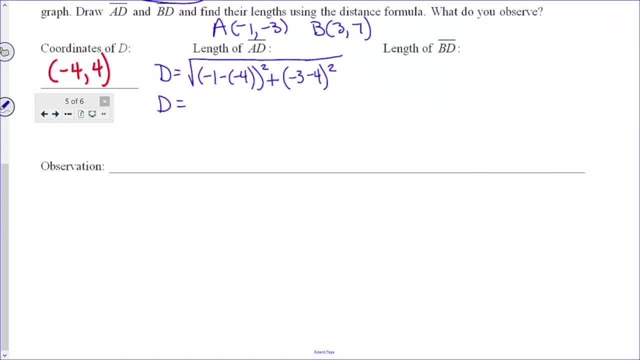 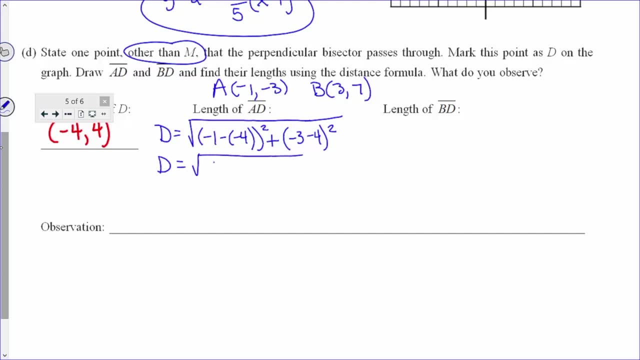 Let me keep going. Let me extend my page a little bit so I have an easier time writing. Negative 1 minus negative 4.. Be careful, Right, That's going to be a positive 3 squared. Negative 3 minus 4 is negative 7 squared. 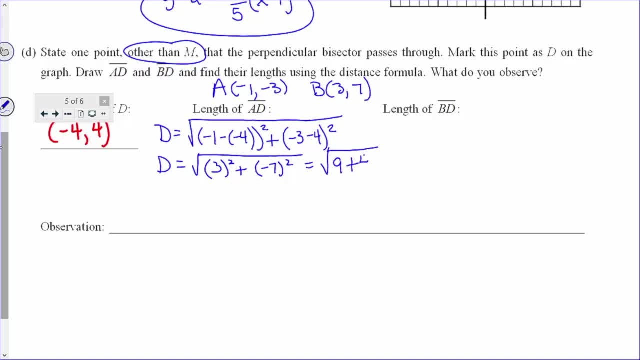 All right, 3 squared is 9.. Negative 7 squared is 49.. And I get the distance as the square root of 58.. Now, 58 is not a nice, perfect square, All right. So what should I do with this? 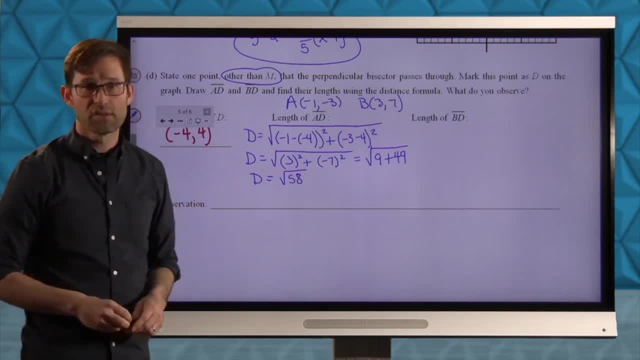 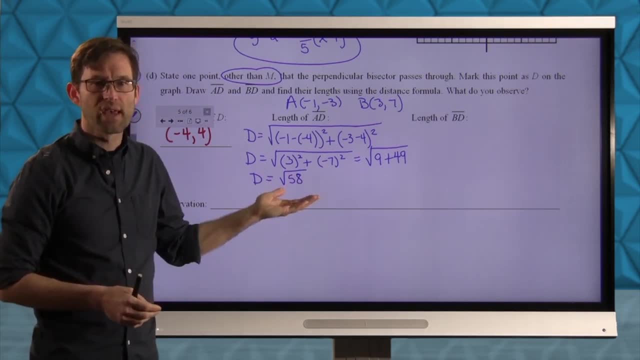 Well, I see no reason to do anything with it other than leave it as the square root of 58.. Just leave it that way. I mean, I could also write it to the nearest tenth, or something like that. But why not leave the answer exact as the square root of 58?? 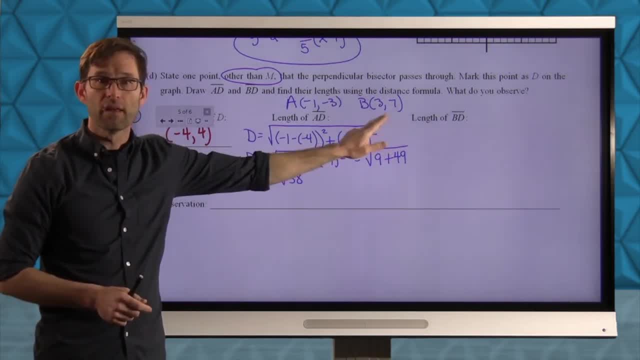 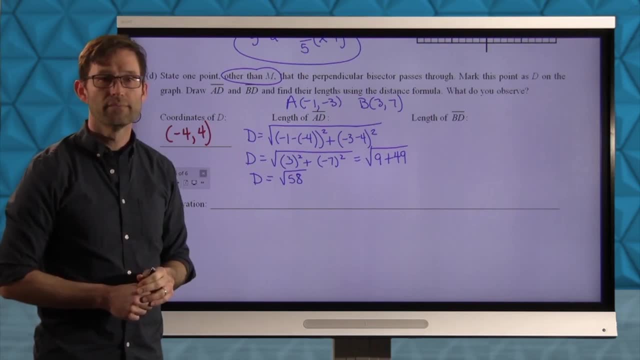 Now what I'd like you to do is work out the length of BD by using point B and point D. Let me move this out of the way. All right, Take a few minutes to do that. All right, Let's go through. 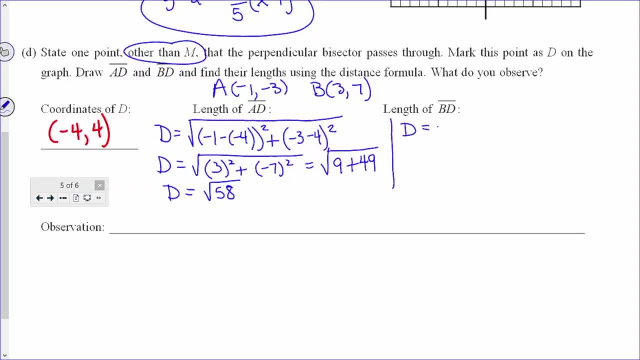 Again, just using the distance formula. The distance is the square root of 3.. Minus negative 4 squared plus 7 minus 4 squared- All right, 3 minus negative 4, be careful- is 7.. 7 minus 4,- that's easy- is 3.. 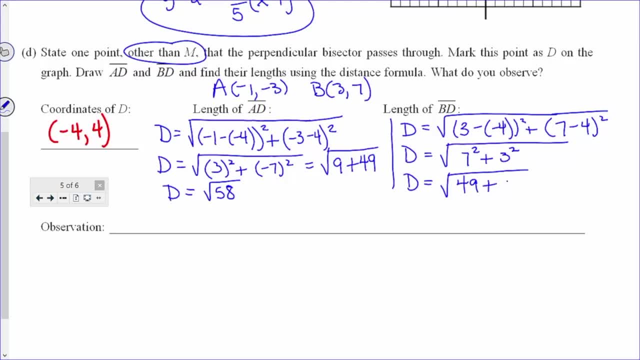 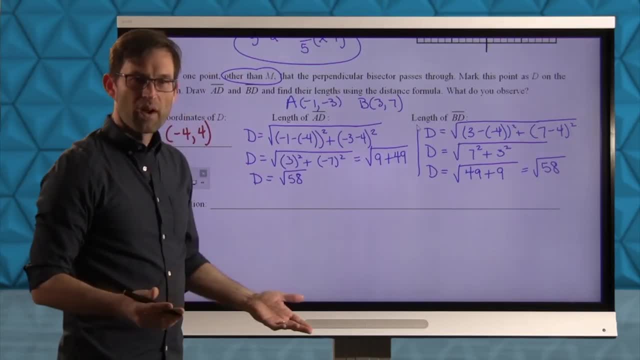 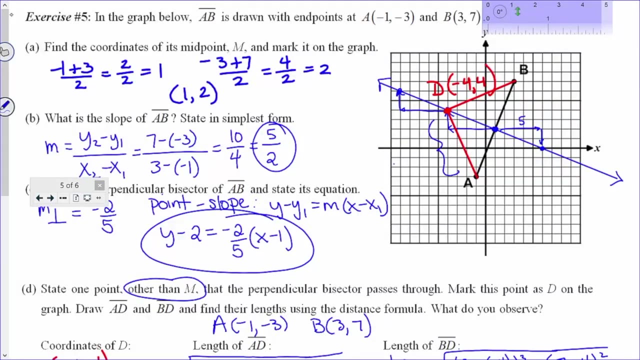 7 squared is 49.. 3 squared is 9.. And I get the square root of 58.. So what observation can we make? Well, this length is the square root of 58.. This length is also the square root of 58.. 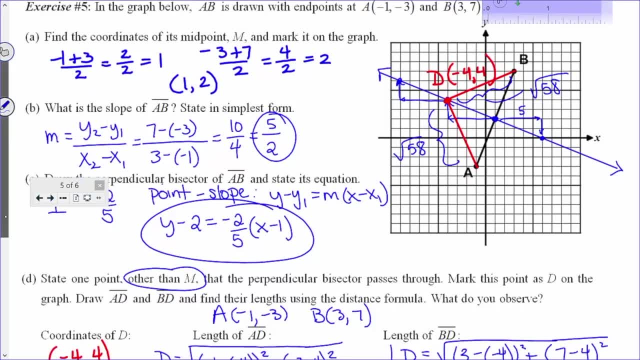 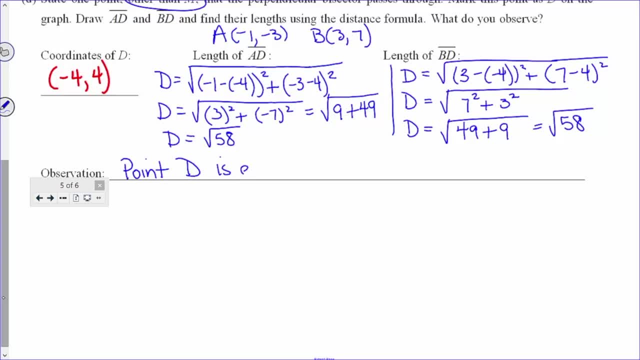 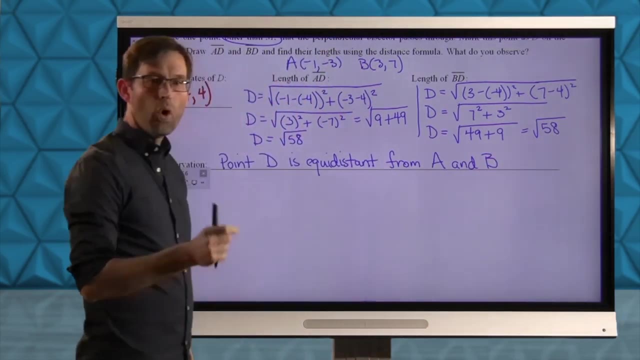 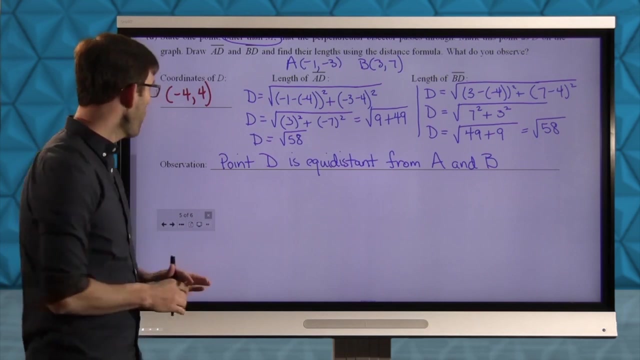 So the observation I can make is that point D is equidistant, So I can get the square root of 58 from A and B, And I'm hoping that sounds familiar to you right. Time and time again we've talked about the fact that any point, any point that lies on 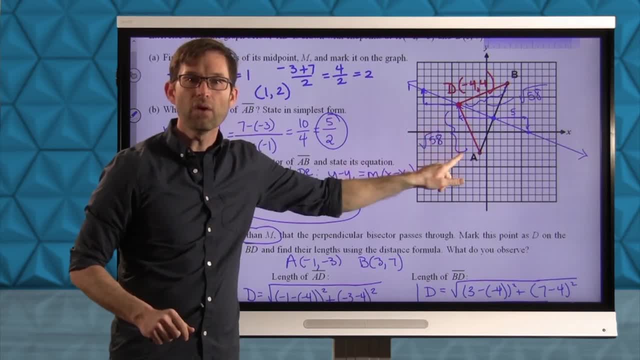 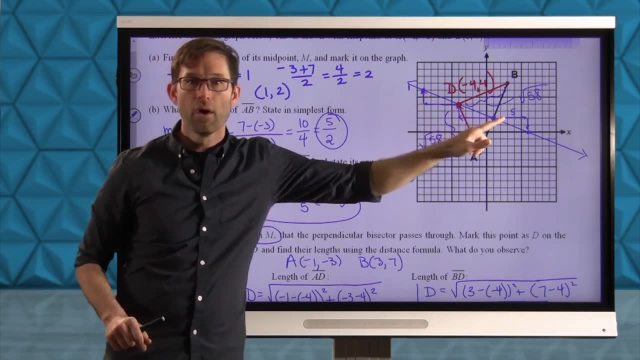 the perpendicular bisector of a line segment should be equidistant from the two endpoints of that line segment. Now I pulled off point D here, But I can't do that. I can't do that. I could have pulled off this point or I could have taken this one down here. 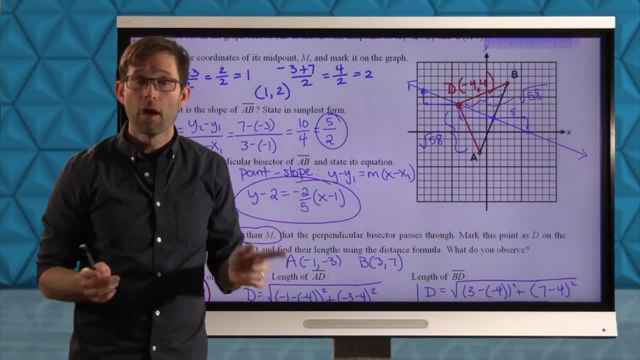 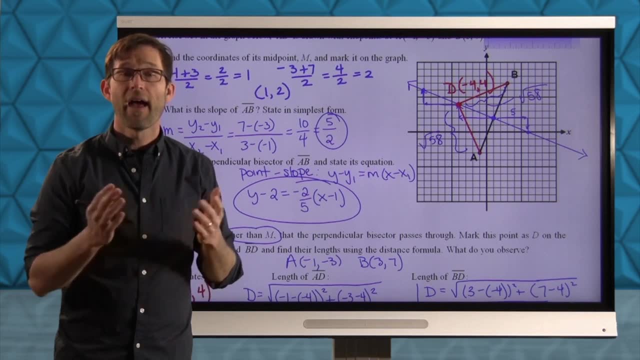 In each case, we wouldn't have found the square root of 58,, but we would have found that both of those line segments, AD and BD, were the same length, hence proving something, or at least showing or illustrating something that we already knew to be true. 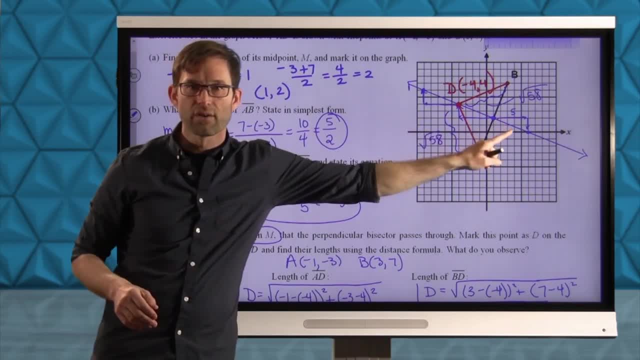 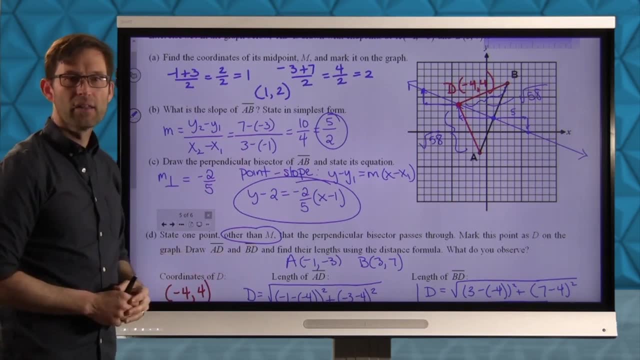 Any any point along that perpendicular bisector will be equidistant from points A and B. All right, let me step back a little bit. allow you some time to copy down anything here you need to. Let me pull the page down a little bit. 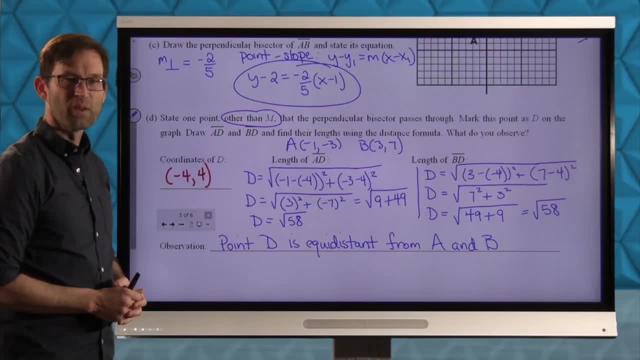 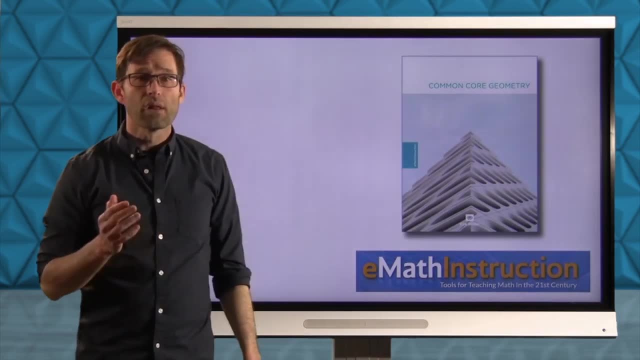 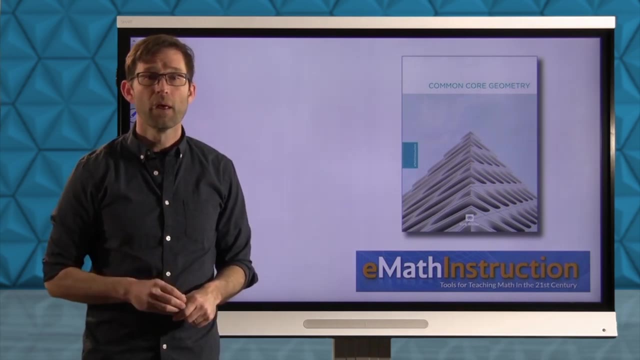 Anything here? Okay, and let's wrap up Okay. So today, what we saw was the last of the three major formulas that we need in coordinate geometry. Those three formulas are the slope formula, the distance formula and the midpoint formula.